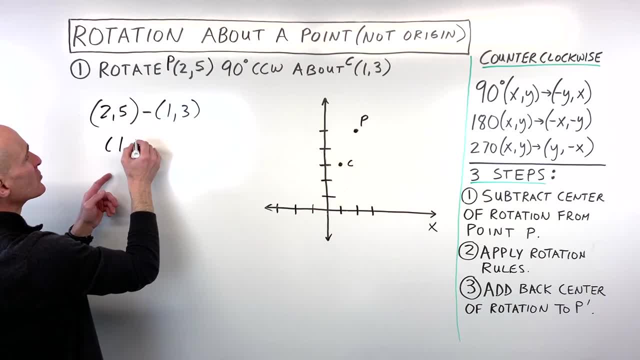 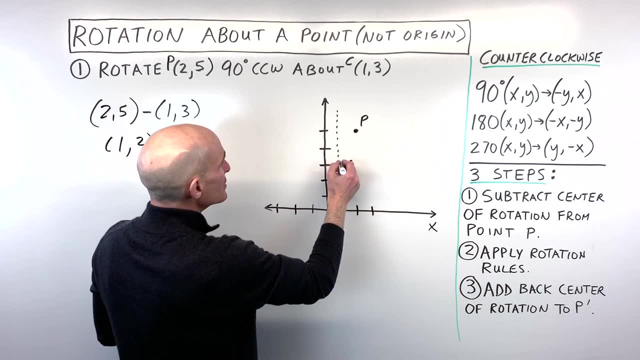 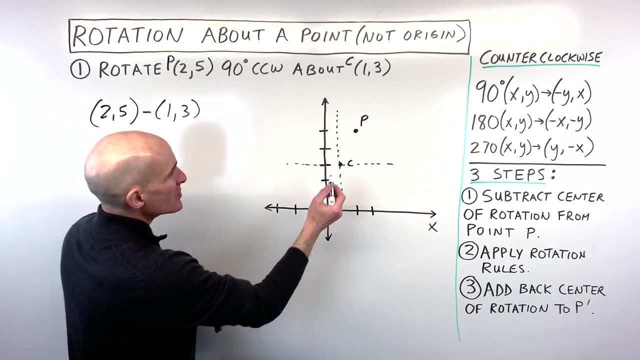 and two minus one comes out to one, and five minus three comes out to two. Now you're probably saying, well, why are we doing that, right? Well, imagine if your center of rotation is like your new origin. Okay, so I'm drawing in a dash: x and y axis. there You can see. point P is really like right one. 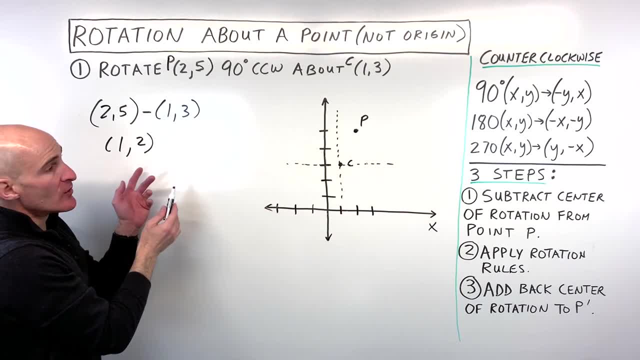 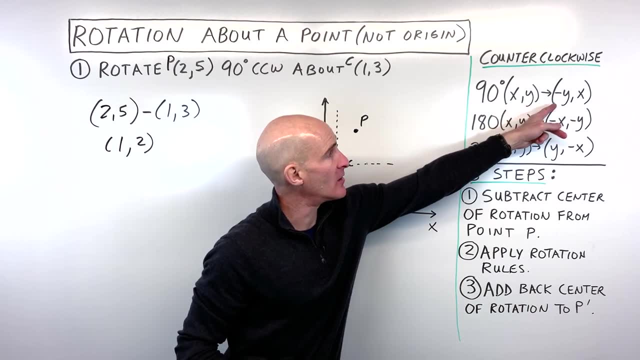 up two. See how we have one comma two. So now what we're going to do is we're going to apply our rotation rules. In this case, 90 degrees, counterclockwise x y becomes negative y x. So the way I like to think about it is: you switch the x and the y. 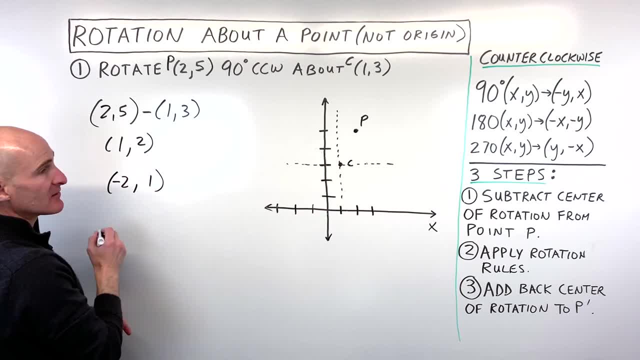 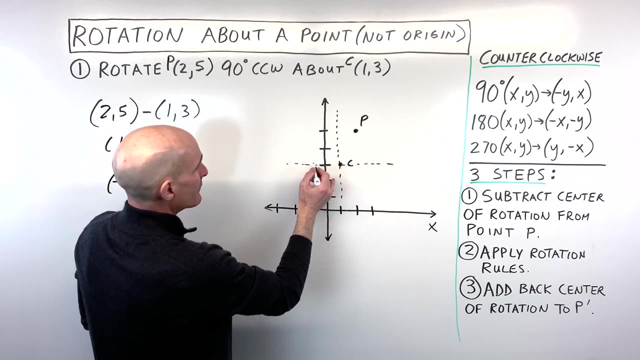 and you make this new x value the opposite sign. Okay, that's how I like to think about it. You switch the x and the y. the new x becomes the opposite. Okay, so now we're at negative 2, comma 1.. So from this perspective you can think about. this is like left two up one, and you can see how we've. 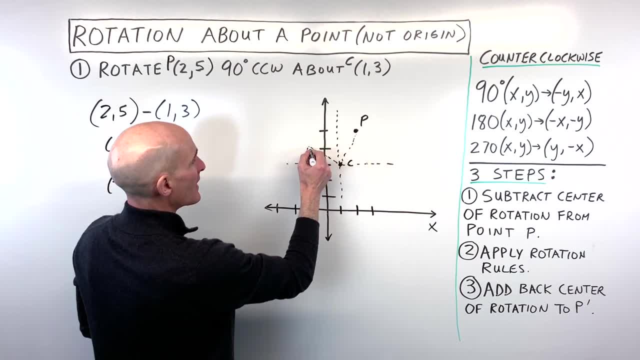 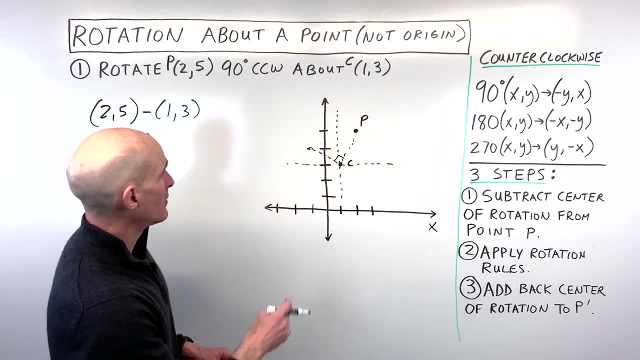 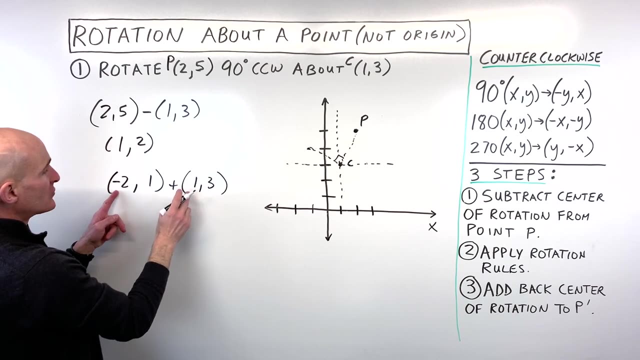 rotated that 90 degrees. I'll even draw on some more dotted lines, see that right angle. But then what you want to do is you want to add back the center of rotation to this new point: negative 2: 1.. So if we do that, our center of rotation is one comma three Negative two plus one is negative one. 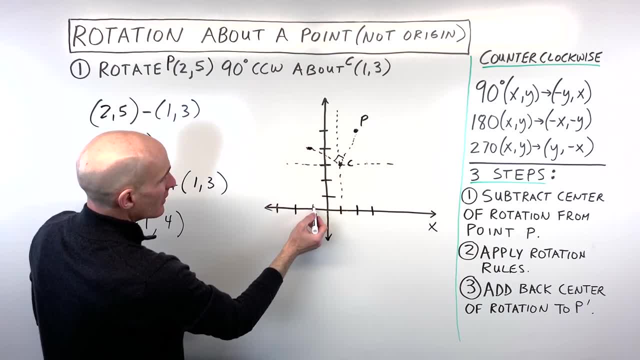 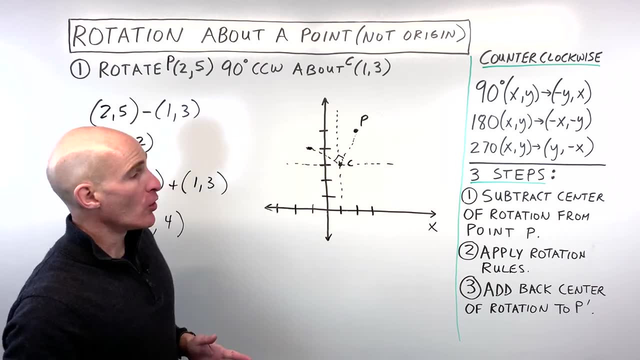 is four And look at where this point is right. here You're at left, one up four, And that's exactly where the point is located. So three easy steps. Let's try another example. See if you can practice this one on your own. Okay, example number two: See if you can pause the video and try this. 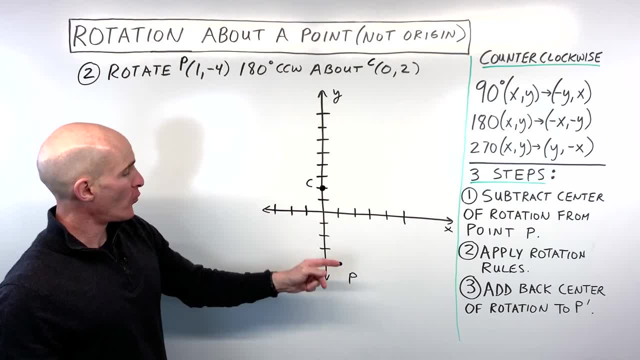 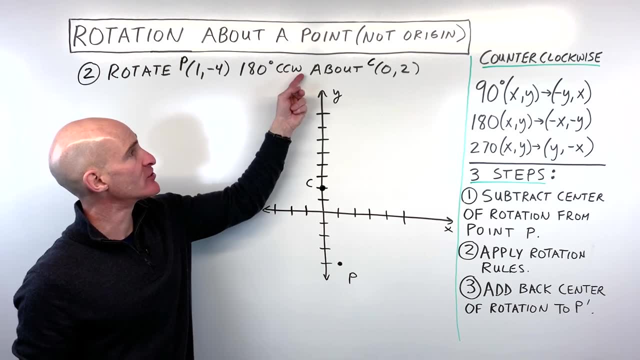 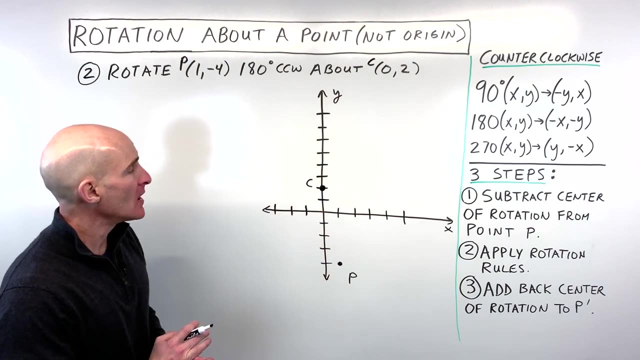 one on your own. We're rotating this point one negative four, 180 degrees, counterclockwise or clockwise doesn't matter, because 180 is a half rotation, half turn About the center, new center of rotation, which is at zero comma two right here. So go ahead and try that one. 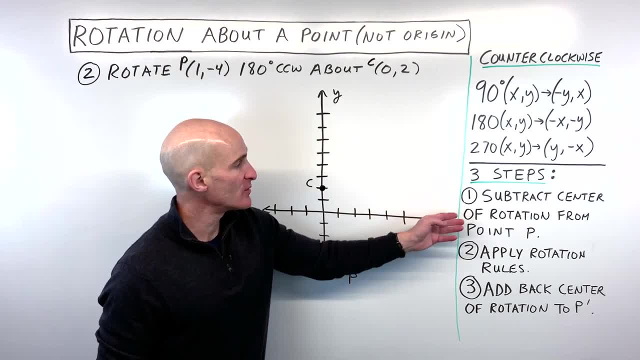 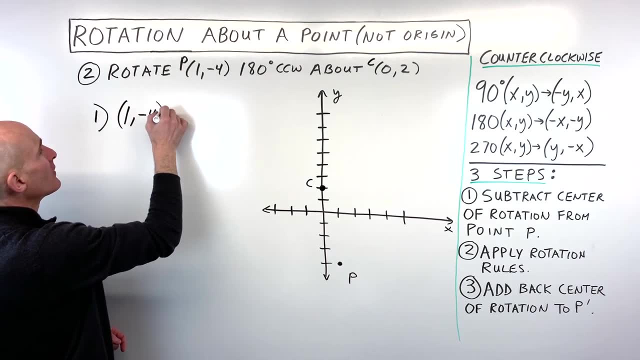 Now, if I was going to do it, what I would do is apply these rules. The first thing would be to subtract the center rotation from our point. So I'll just label these steps. So, step one: we take one negative four and we subtract zero, comma two, So that's going to give us one minus. 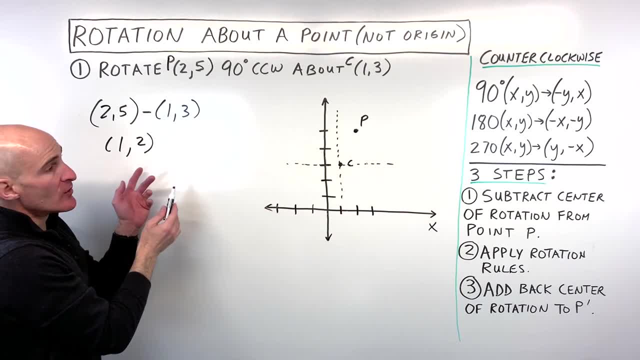 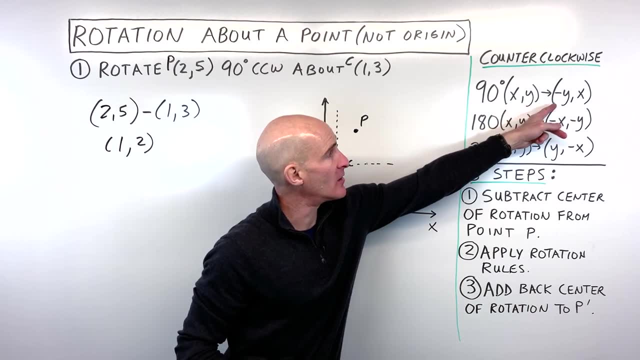 up two. See how we have one comma two. so now what we're going to do is we're going to apply our rotation rules. in this case, 90 degrees, counterclockwise x y becomes negative y x. so the way I like to think about it is: you switch the x and the y. 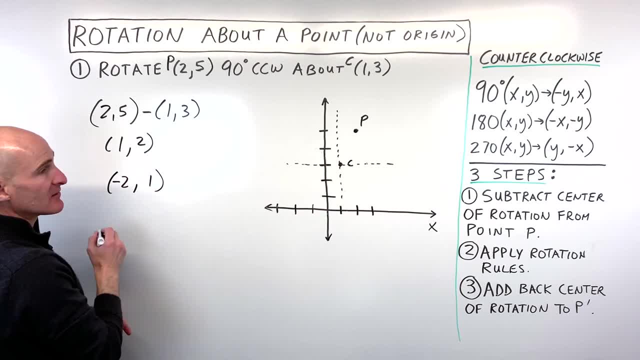 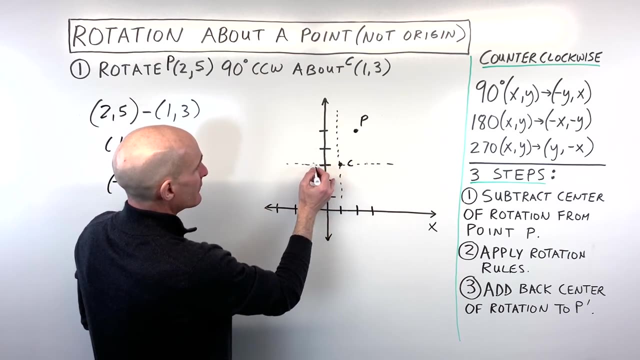 and you make this new x value the opposite sign. Okay, that's how I like to think about it. You switch the x and the y and the new x becomes the opposite. Okay, so now we're at negative two comma one. So from this perspective you can think about this is like: left 2, up 1, and you can see how we've rotated that 90 degrees. 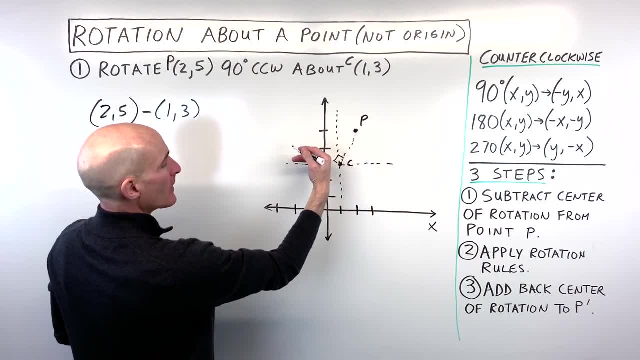 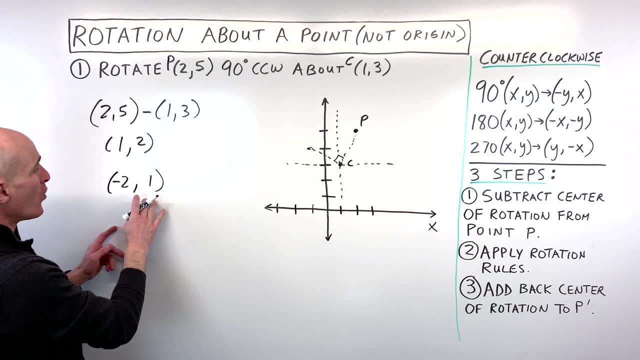 I'll even draw on some more dotted lines, see that right angle. But then what you want to do is you want to add back the center of rotation to this new point: negative 2, 1.. So if we do that, our center of rotation is 1, 3, negative 2 plus 1 is negative 1, and 1 plus 3 is 4.. 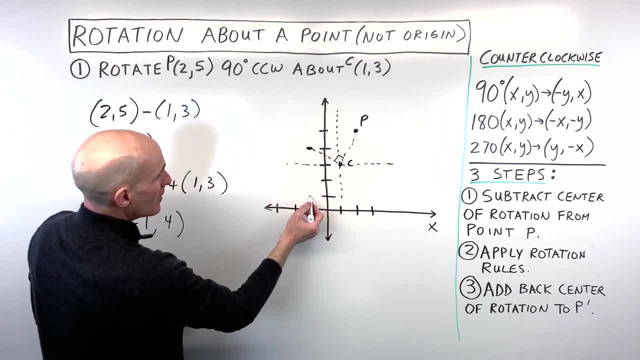 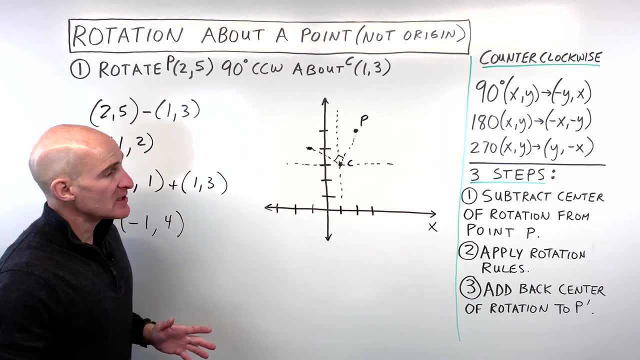 And look at where this point is right. here You're at left 1, up 4, and that's exactly where the point is located. So three easy steps. Let's try another example. See if you can practice this one on your own. 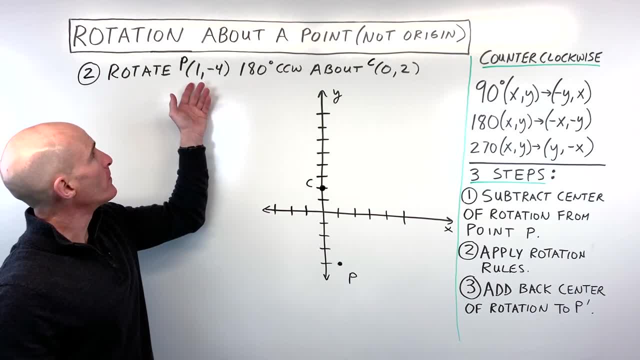 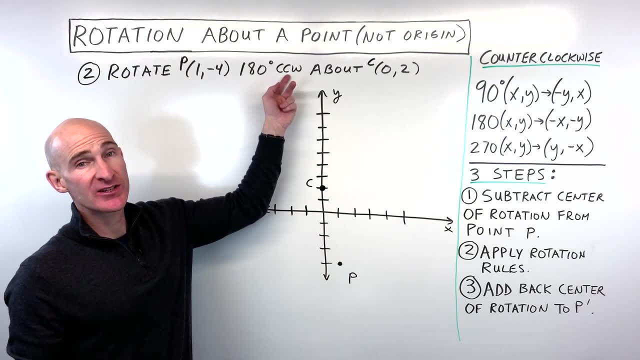 Okay, example number two. See if you can pause the video and try this one on your own. We're rotating this point 1, negative 4.. 180 degrees, counterclockwise or clockwise, it doesn't matter, because 180 is a half rotation, half turn. 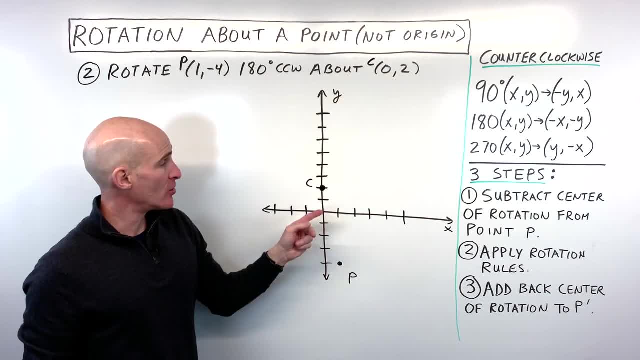 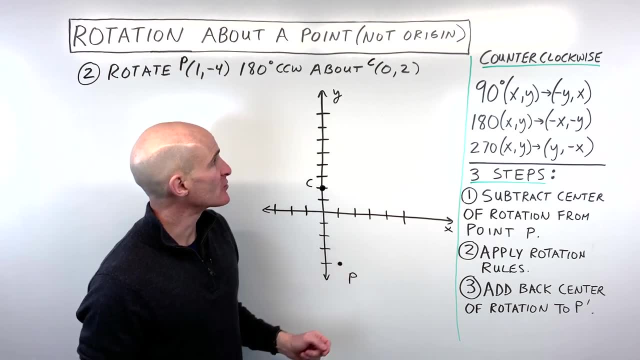 about the center, the new center of rotation, which is at 0, 2 right here. So go ahead and try that one Now. if I was going to do it, what I would do is apply these rules. The first thing would be to subtract the center of rotation from our point. 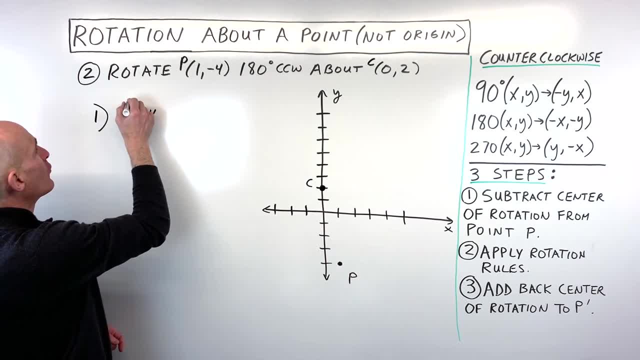 So I'll just label these steps. So step one: we take 1, negative 4, and we subtract 0,, 2.. So that's going to give us 1.. 1 minus 0 is 1, and negative 4 minus 2 is negative 6.. 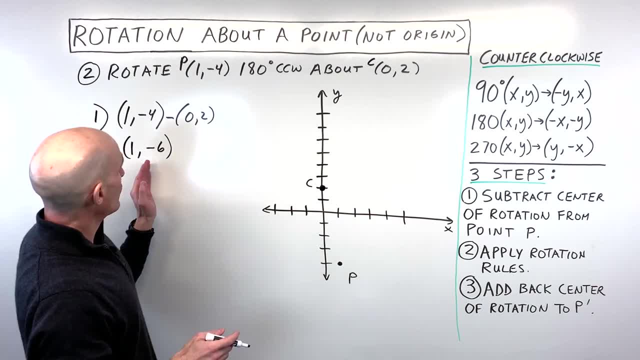 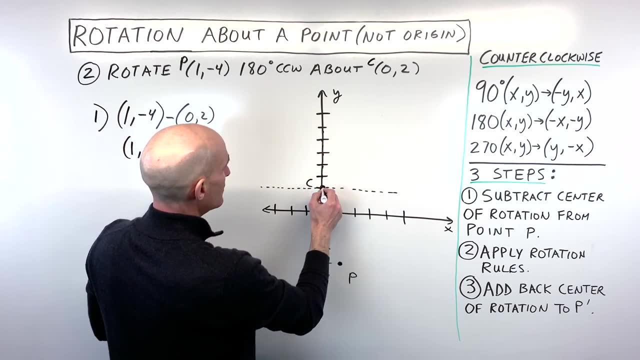 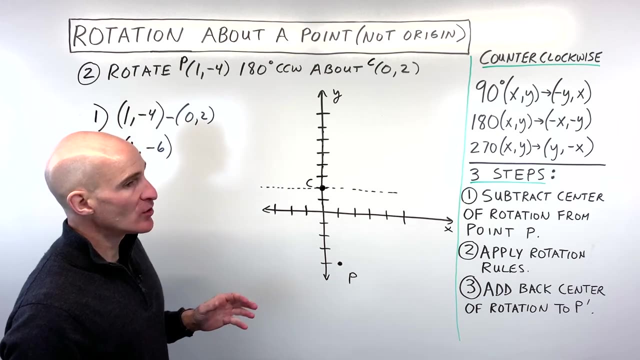 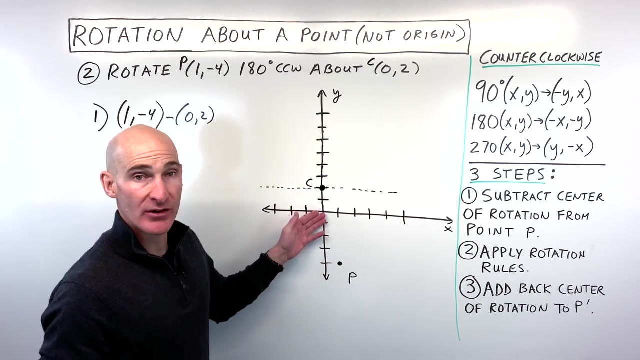 Now to try to understand this. you know a little bit more deeply. we can think about the center of rotation as like our new origin, right. So we kind of have a new origin point right there And when we're subtracting 0,, 2, okay, what that's basically doing is it's taking the center of rotation and it's moving it back to where the origin is. 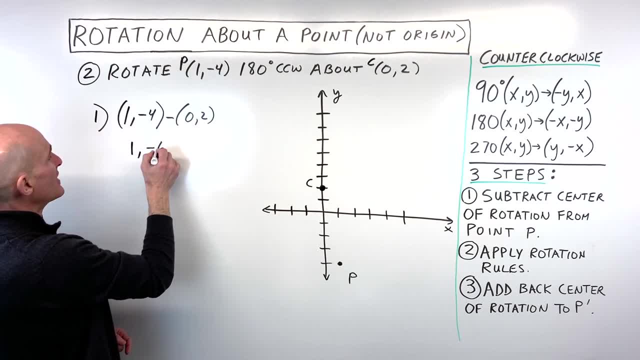 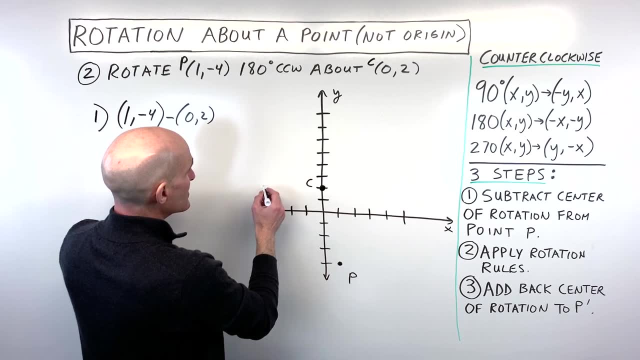 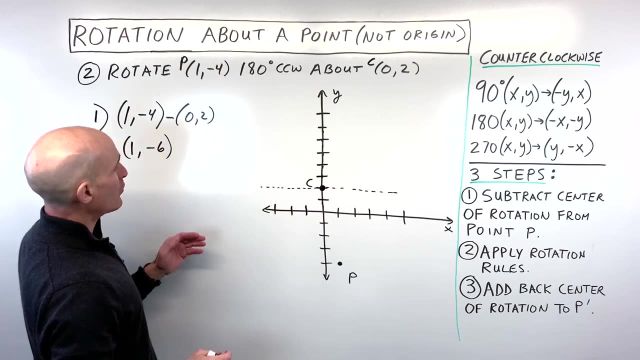 zero is one and negative four minus two is negative six. Now, to try to understand this, you know a little bit more deeply. we can think about the center of rotation as like our new origin right. So we kind of have a, a new origin point right there And when we're subtracting zero, two, okay, what that's basically. 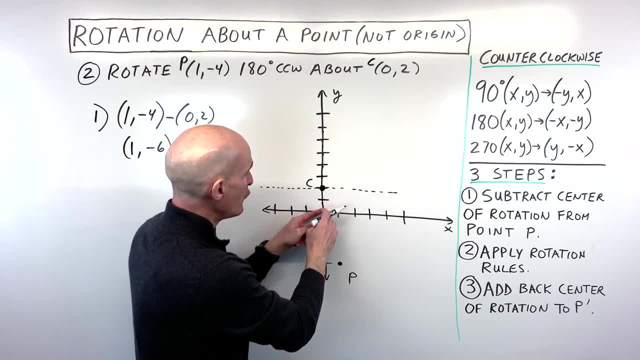 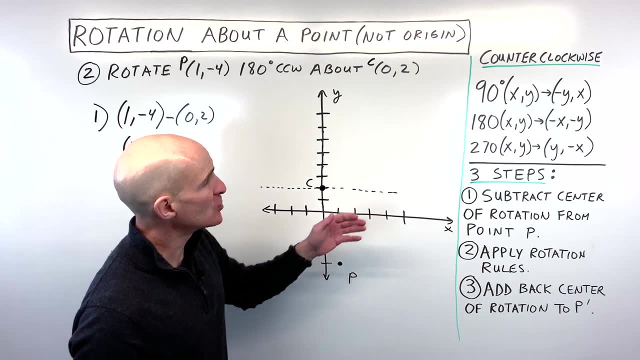 doing is it's taking the center of rotation and it's moving it back to where the origin is- Okay, where our normal origin is, And so, then, what that allows us to do is to apply our rules, just like we normally do when we're rotating about the origin. So you can see this point one. 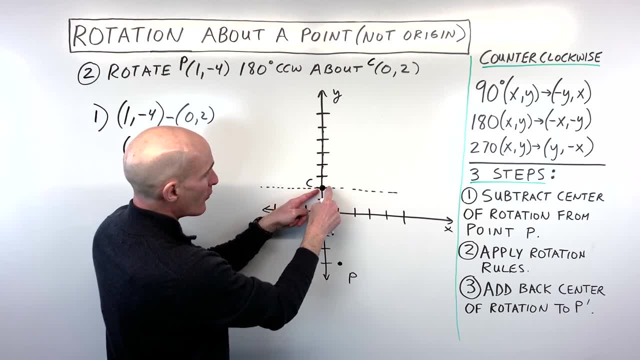 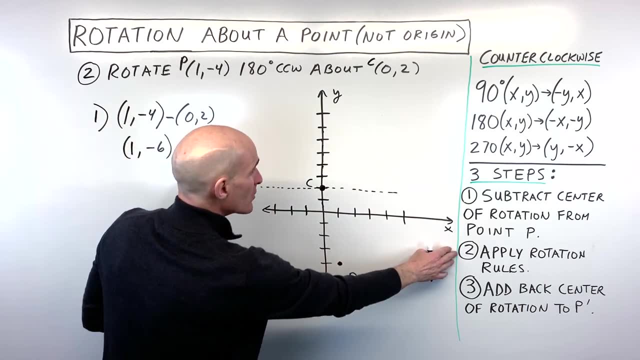 negative six. from the perspective of this new center rotation, we're at right one down six. See, there's our point, as if that was the the origin right. So then, step number two is we're going to apply the rotation rules Now with 180 degrees. all we do is we keep the x and the y in the same order. 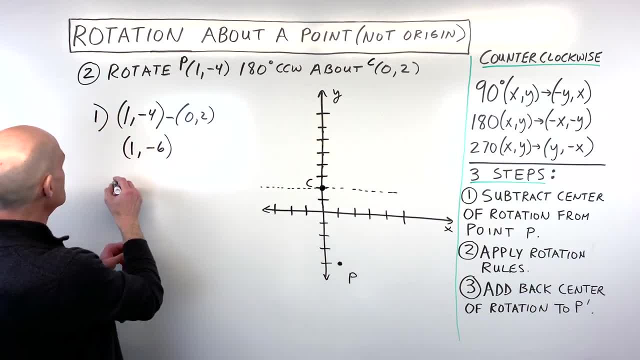 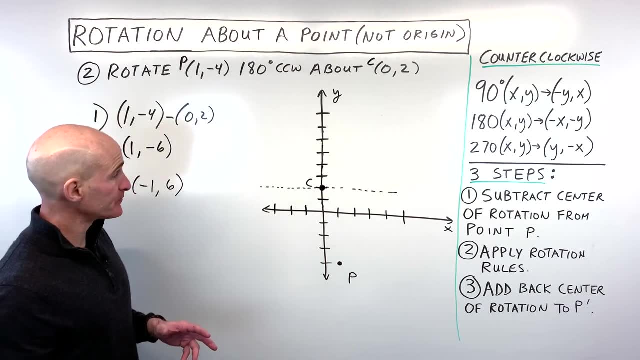 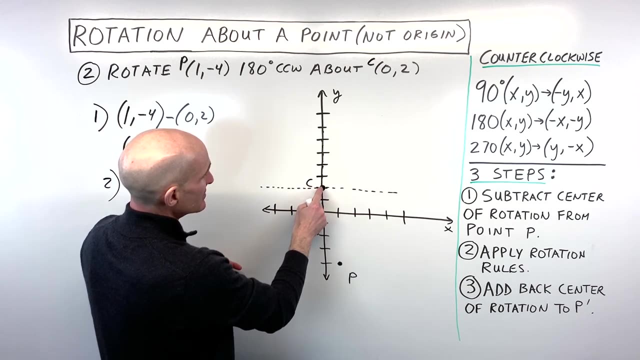 but we make them the opposite sign. Okay, so what that's going to be is now for step two. this will become negative one, this will become positive six. so the signs flip. So negative one, six is going to be negative one, and negative one is going to be negative one. So what does that mean? 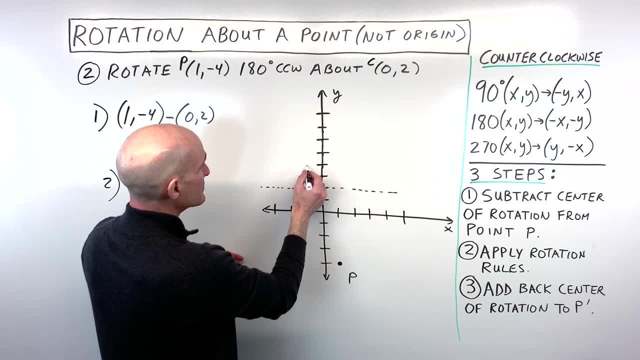 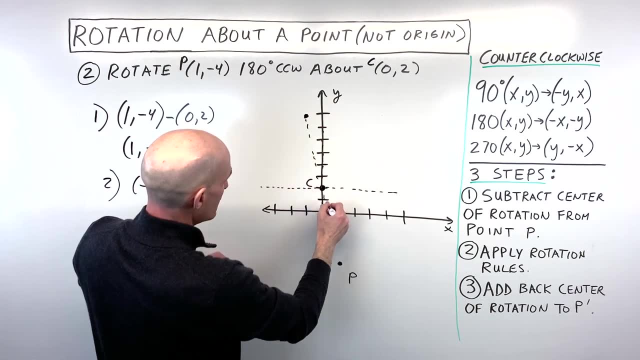 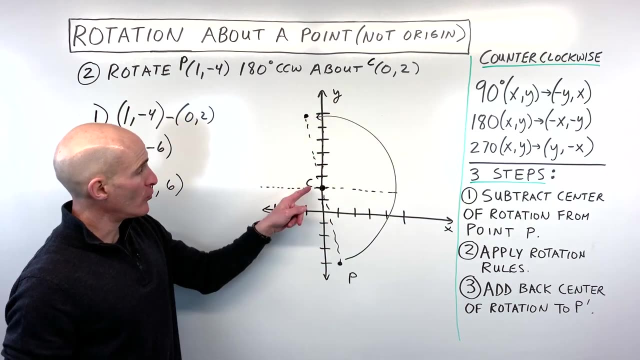 Well, basically what it means is that from this center of rotation, this new point, if we were to go left one up six, that would put us right here. So you're basically turning. let me see if I can draw a dotted line here. you're doing like a half turn and you can see this point is ending up right. 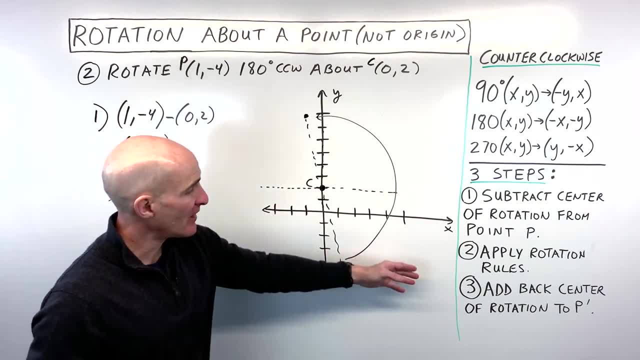 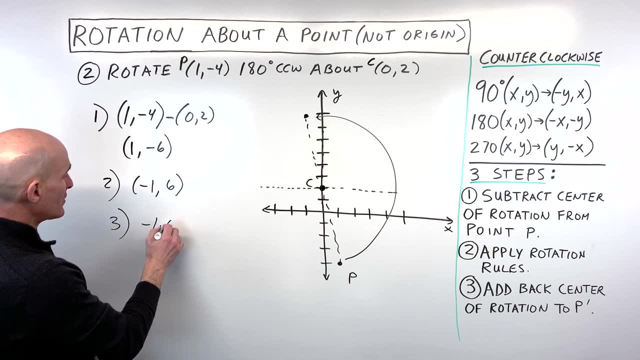 there rotating or pivoting about this new center of rotation, right, But then what's going to happen is we're going to add back that center of rotation to that point. So for step three we're going to take negative one, six, we're going to add back zero, comma two, So negative one plus zero is negative. 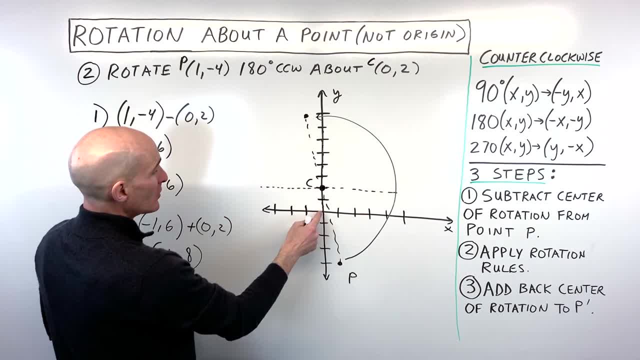 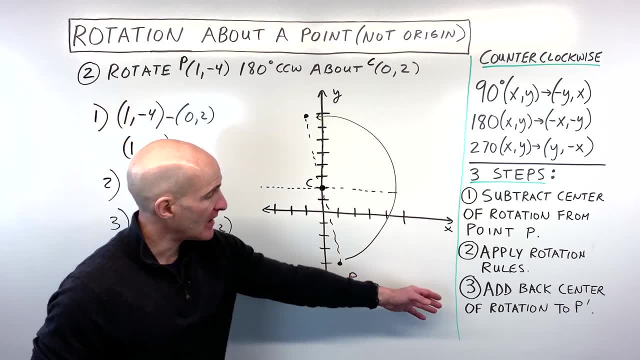 one and six plus two is eight, And you can see that that's where our point is located. from the original zero zero point, the original origin left one up eight. Now why are we adding back that center of rotation at the very end there? Well, remember, originally we subtracted it. Okay, so the 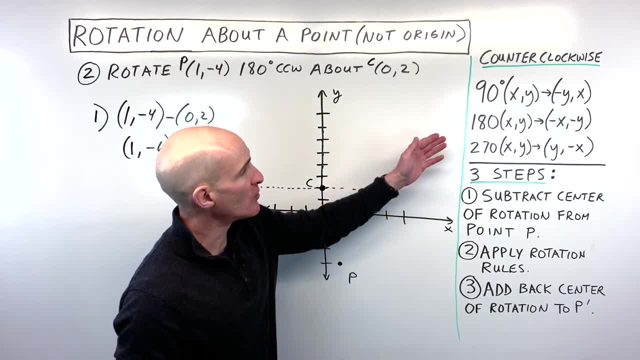 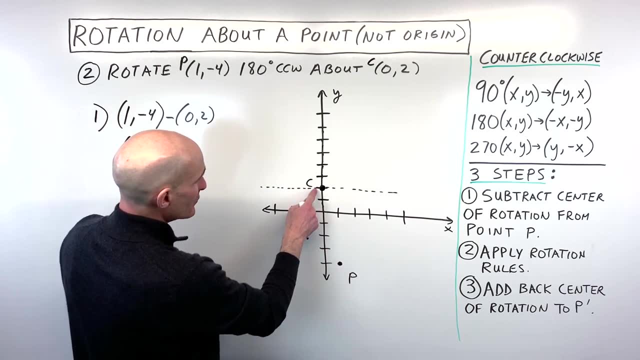 Okay, And so then, what that allows us to do is to apply our rules, just like we normally do when we're rotating about the origin. So you can see this point 1, negative 6, from the perspective of this new center of rotation. we're at right 1, down 6.. 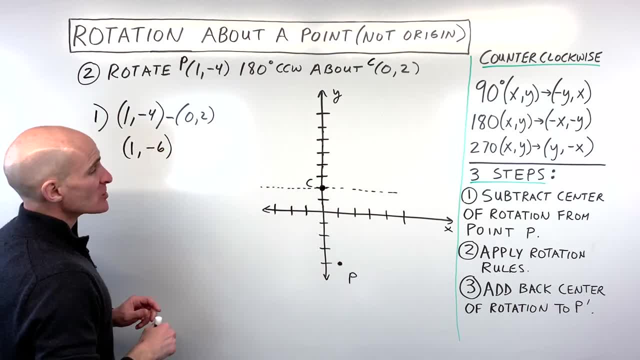 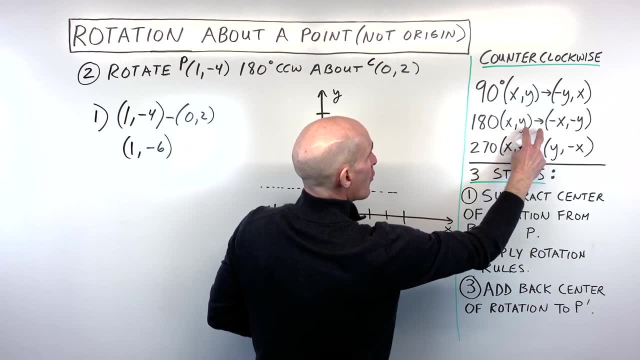 See, there's our point, as if that was the origin, right. So then, step number two is we're going to apply the rotation rules Now with 180 degrees. all we do is we keep the x and the y in the same order, but we make them the opposite sign. 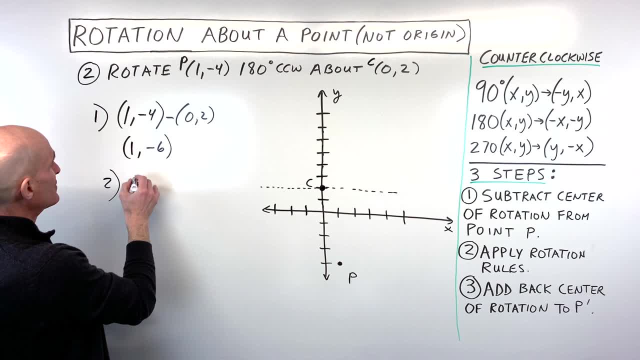 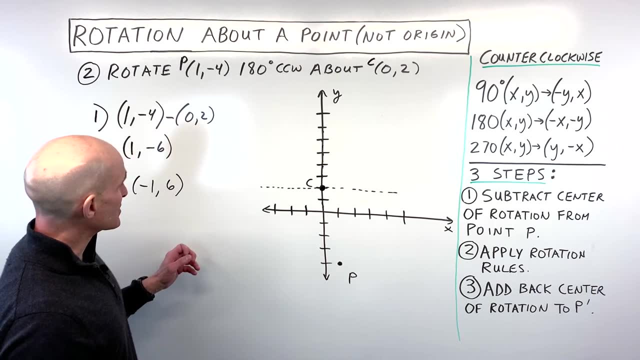 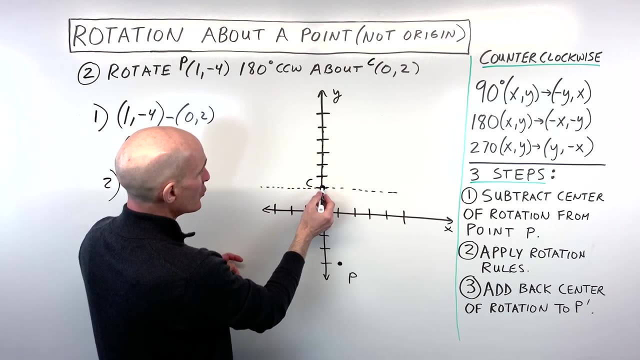 Okay, So what that's going to be is Now for step two. this will become negative 1,, this will become positive 6, so the signs flip. So negative 1, 6, what does that mean? Well, basically, what it means is that from this center of rotation, this new point, if we were to go left 1, up 6, that would put us right here. 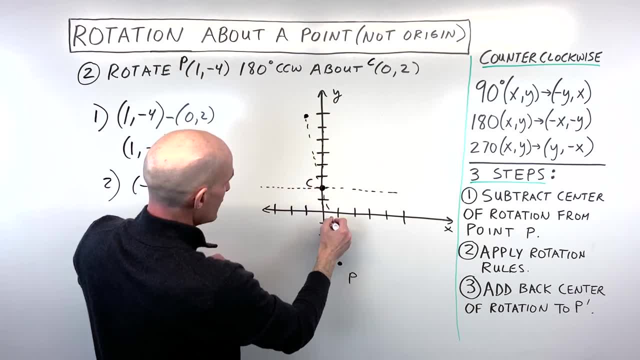 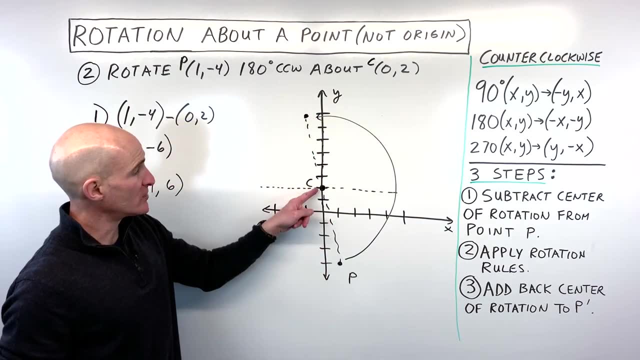 So you're basically turning. let me see if I can draw a dotted line here. you're doing like a half turn and you can see this point is It's ending up right there rotating or pivoting about this new center of rotation, right? 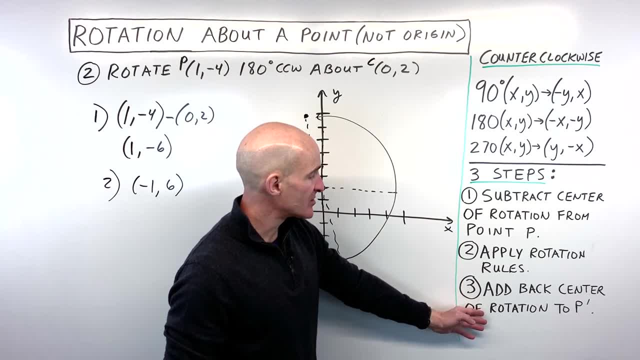 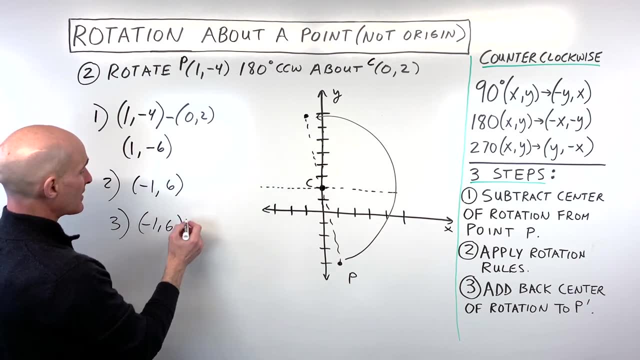 But then what's going to happen for the last step is we're going to add back the center of rotation to that point. So for step three, we're going to take negative 1, 6, we're going to add back 0, 2.. 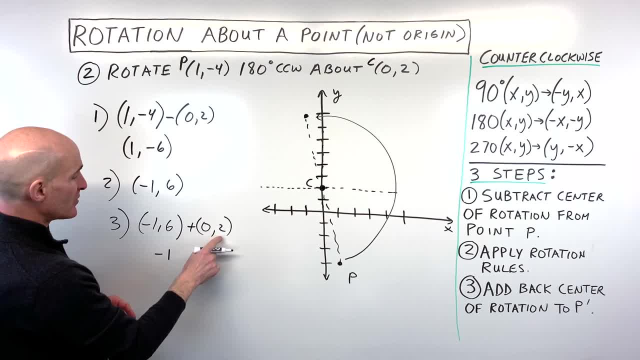 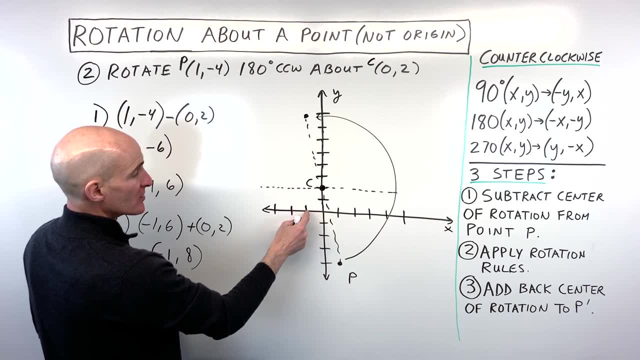 So negative 1 plus 0 is negative 1, and 6 plus 2 is 8.. And you can see that that's where our point is located from the original 0, 0 point, the original origin Left 1.. 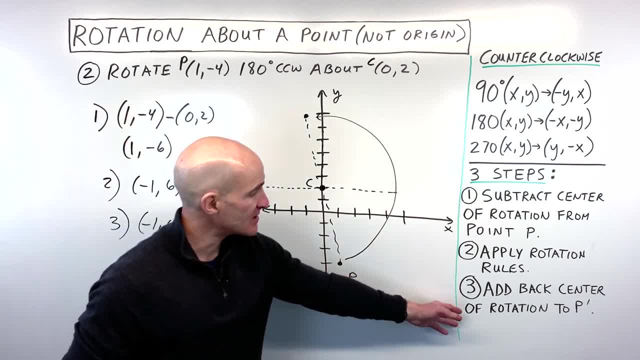 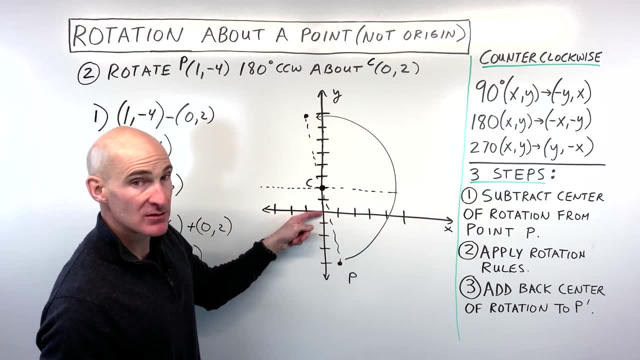 Up 8.. Now why are we adding back that center of rotation at the very end there? Well, remember, originally we subtracted it. okay, So that basically brought this point to the origin. Now, when we add it back, we're putting it back to where we started, right? 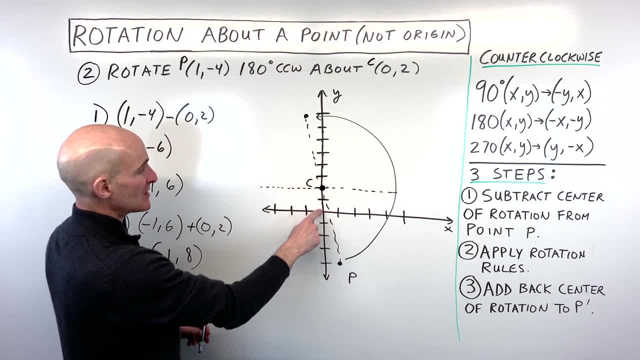 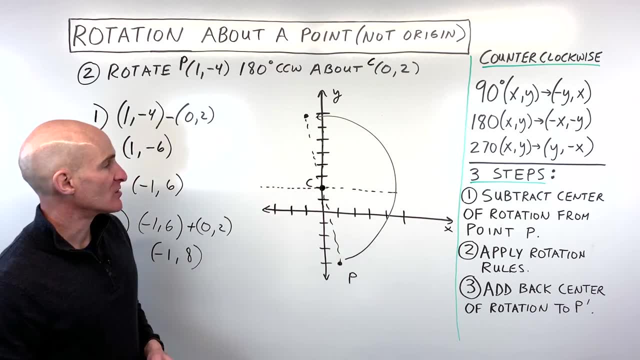 So it's just like a translation, Like if you're sliding everything down to, which is what we did here originally, then we rotated, then we had to move everything back up to to put it into the final position there. So let's try one more example. 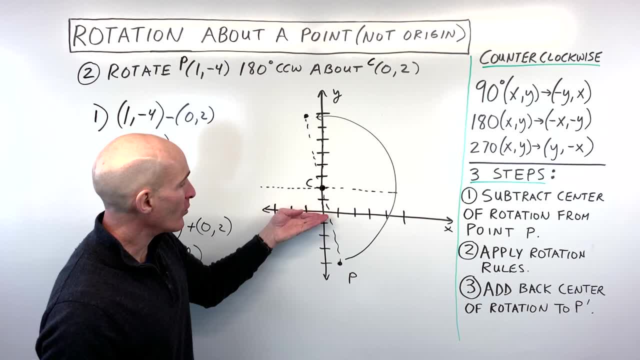 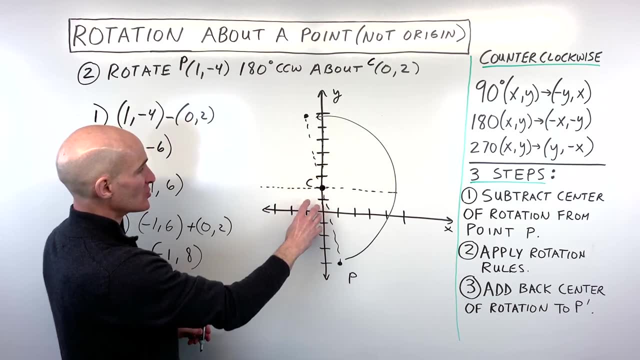 that basically brought this point to the origin. Now, when we add it back, we're putting it back to where, to where we started, right. So just like a translation, like if you're sliding everything down to, which is what we did here originally, then we rotated, then we had to move everything back up to. 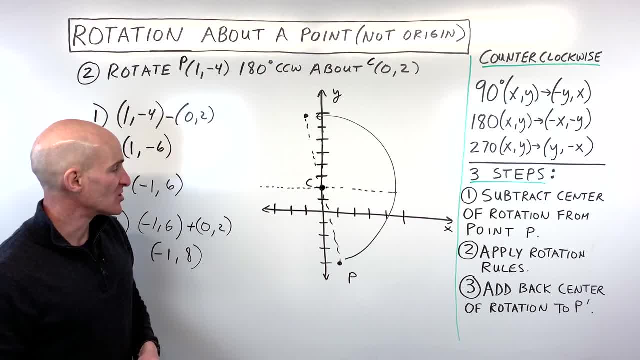 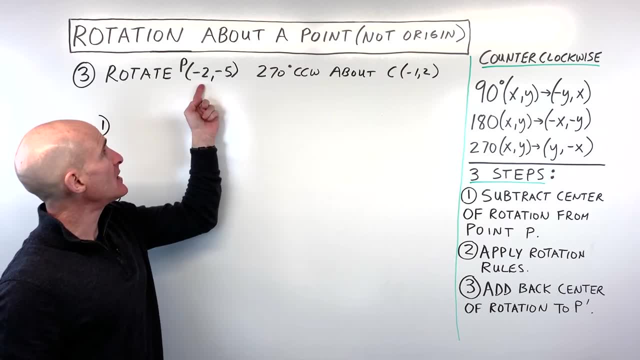 to put it into the uh, you know, to the final position there. So let's try one more example. Okay, see if you can pause the video and try example number three, This one: we're rotating point p, negative two negative five. two hundred and seventy degrees counterclockwise. 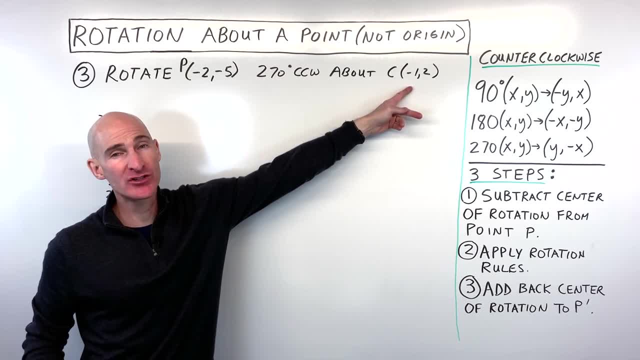 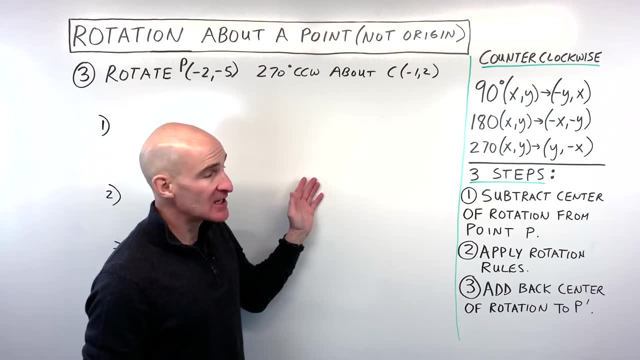 About the new center of rotation here. negative one comma two. This is the point you're pivoting or rotating about. So see if you can do that problem. If I was going to do it, notice I didn't even draw a diagram here. I'm just going to follow the three easy steps here. So the first step: 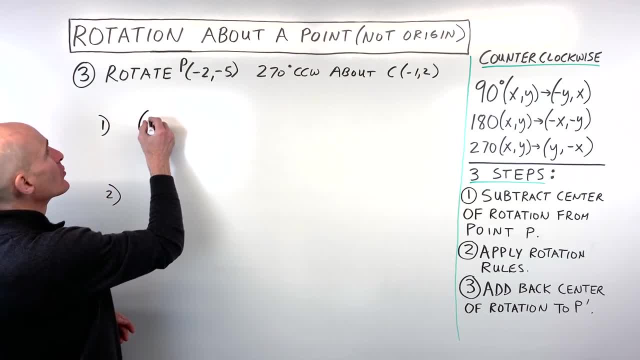 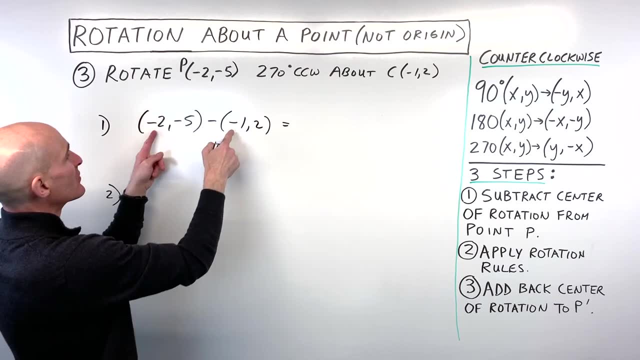 subtract the center of rotation from the point. So we're going to start with negative two, negative five, and we're going to subtract our center rotation. negative one, two, That comes out to negative two. minus negative one is like negative two plus one, So that's negative one. 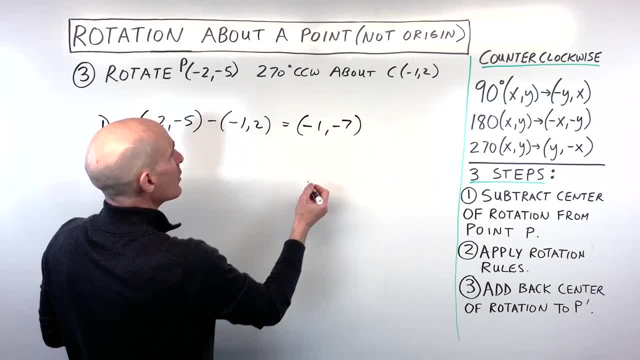 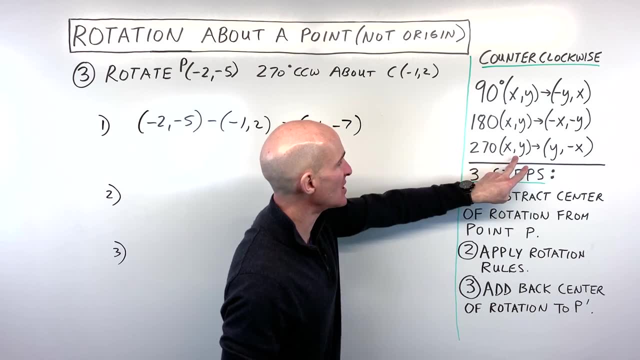 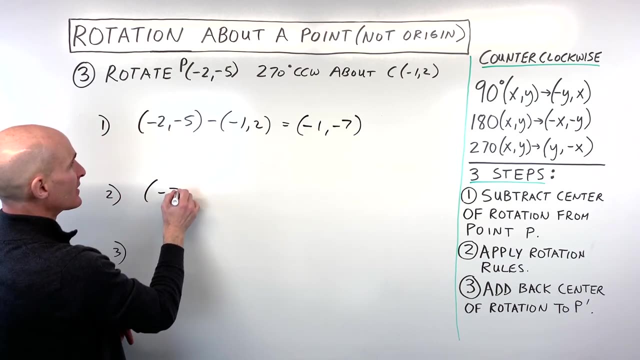 And negative five minus two is negative seven. Okay, good. So now we want to apply the rotation rules For 270. we switch the x and the y, So we basically interchange them and we make the new y value the opposite. So what I mean by that is I switch these, So it's going to become like negative. 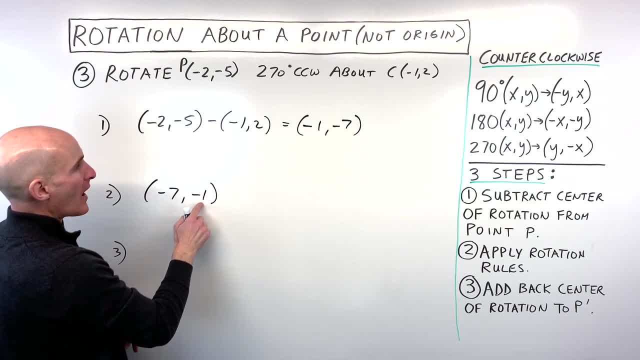 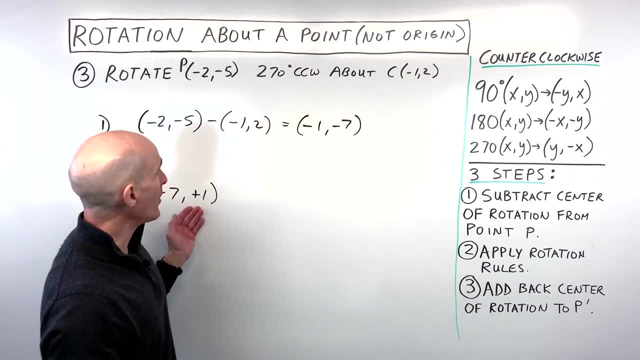 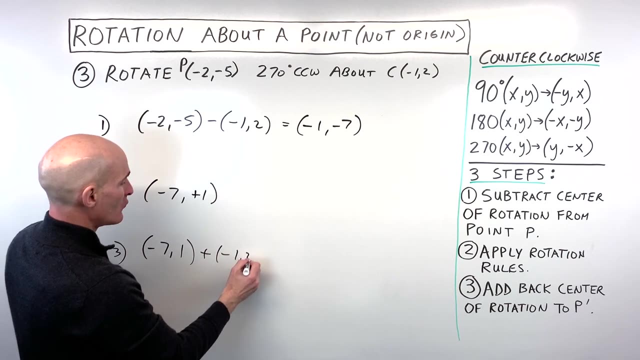 seven, negative one. But I make this new y value the opposite, So that becomes a positive one. Last step is we want to add back that center of rotation to this point. So we're going to say negative seven one plus the new, the center of rotation: negative one, two. 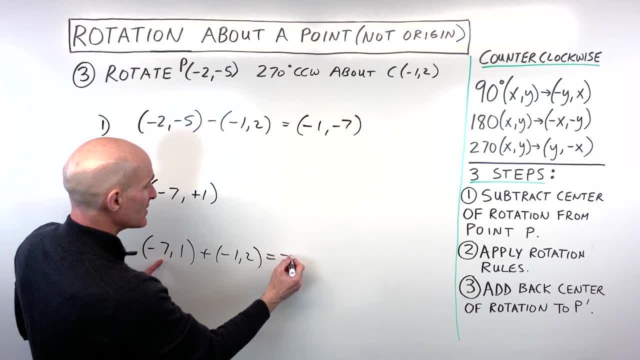 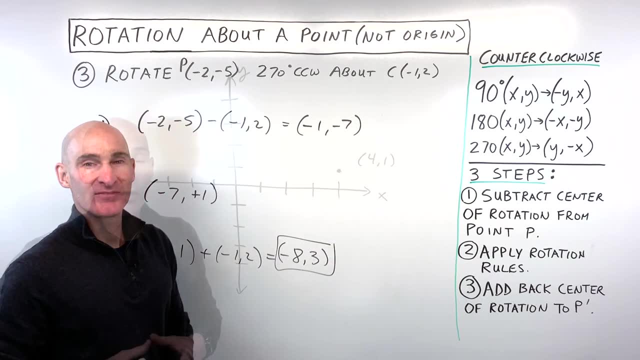 gives us our final location of our point. So negative seven plus negative one is negative eight, and one plus two is three, And you got it Okay. the last thing that I thought we could do together here is just try to understand you know where these uh rules come from, These 90 degree. 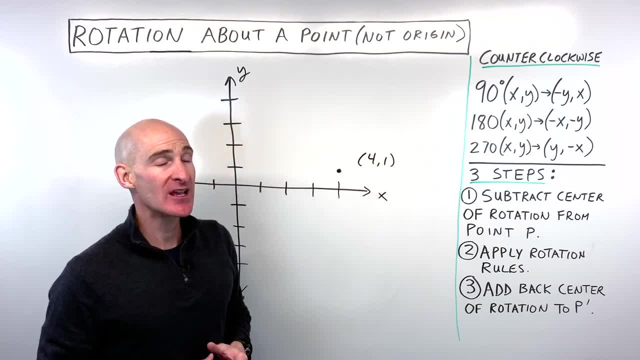 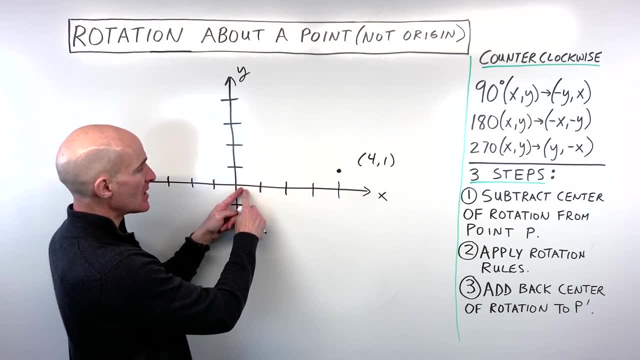 180 degree and 270 degree counterclockwise rotation rules, And so what I'm going to do here, I'm going to take a simple point, and you might want to do this on your own as well, just to kind of visualize. But see if we take this point, 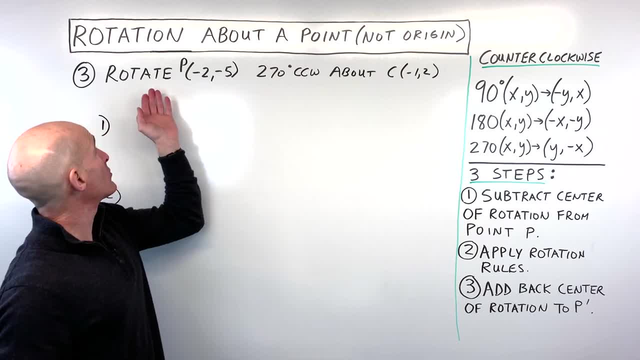 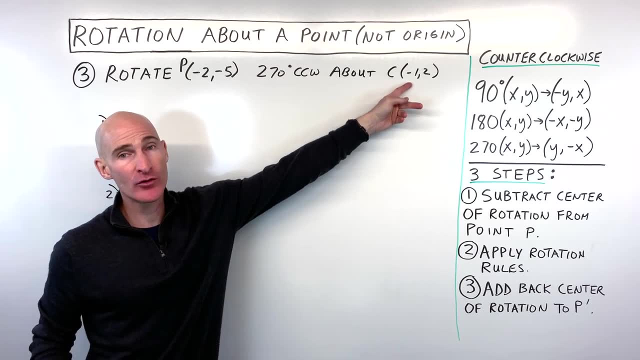 Okay, see if you can pause the video and try example number three, This one: we're rotating point P, negative 2, negative 5, 270 degrees, counterclockwise about the new center of rotation here: negative 1,, comma 2.. 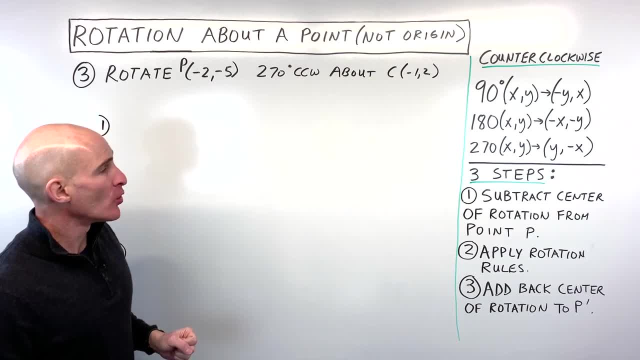 This is the point you're pivoting or rotating about, So see if you can do that problem. If I was going to do it, notice I didn't even draw a diagram here. I'm just going to follow the three easy steps here. 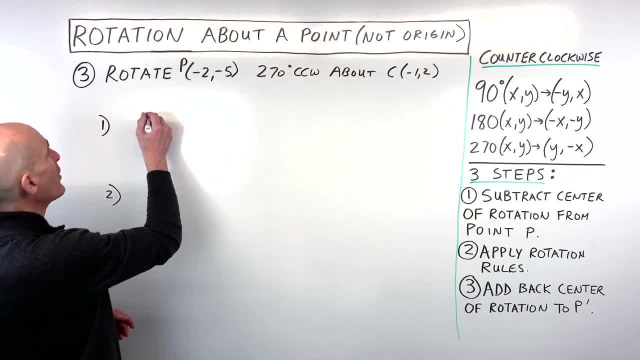 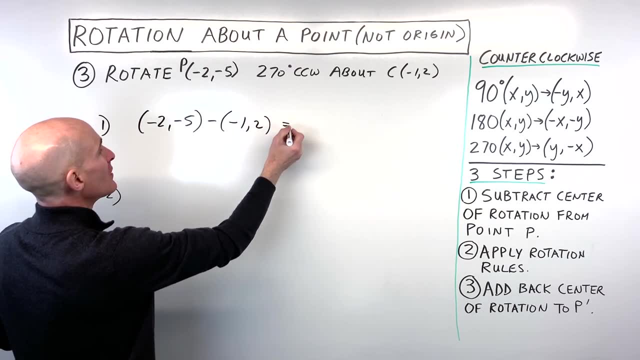 So the first step: subtract the center of rotation from the point. So we're going to start with negative 2, negative 5. And we're going to subtract our center of rotation: negative 1, 2. That comes out to negative 2 minus negative 1 is like negative 2 plus 1.. 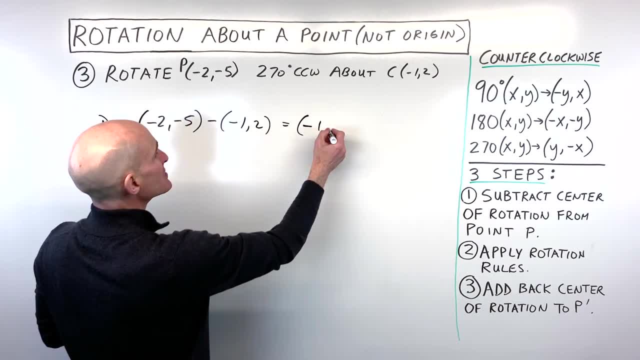 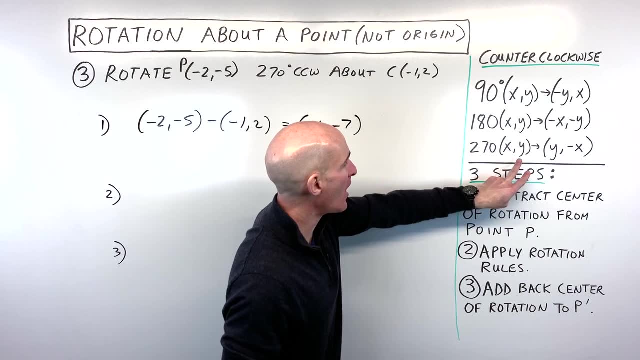 So that's negative 1.. And negative 5 minus 2 is negative 7.. Okay, good. So now we want to apply the rotation rules For 270,. we switch the x and the y, So we basically interchange them. 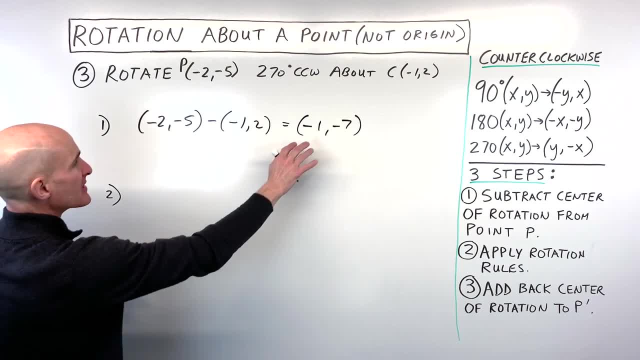 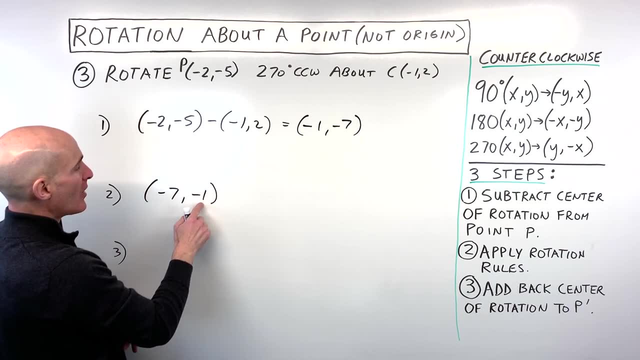 And we make the new y value the opposite. So what I mean by that is I switch these So it's going to become like negative 7, negative 1.. But I make this new y value the opposite, So that becomes a positive 1.. 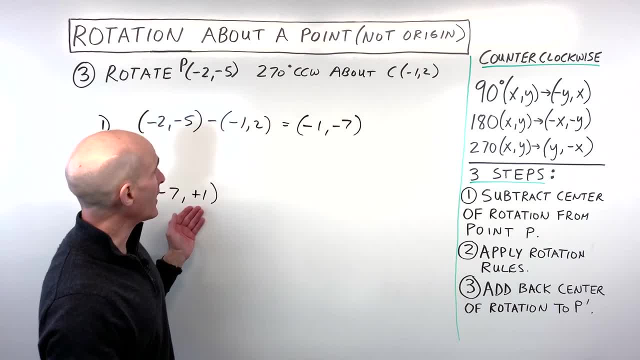 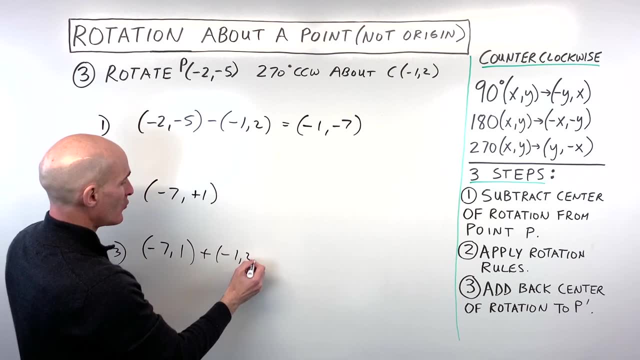 Last step is we want to add back that center of rotation to this point. So we're going to say negative 7, 1 plus the center of rotation, negative 1, 2, gives us our final location of our point. So negative 7 plus negative 1 is negative 8.. 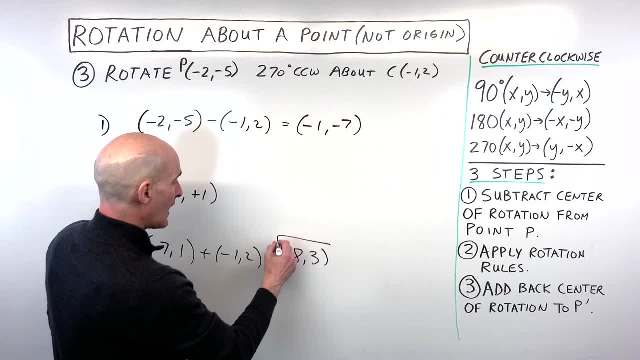 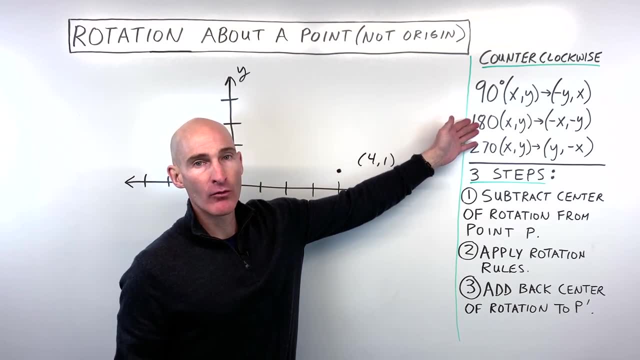 And 1 plus 2 is 3.. And you got it. Okay, the last thing that I thought we could do together here is: just try to understand you know where these rules come from, these 90-degree, 180-degree and 270-degree counterclockwise rotation rules. 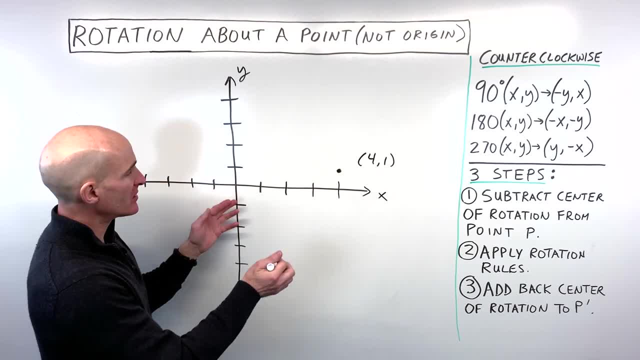 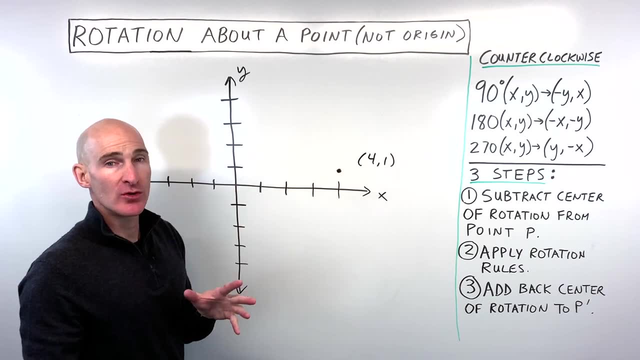 And so what I'm going to do here is: I'm going to take a simple point- And you might want to do this on your own as well- just to kind of visualize. But say, if we take this point 4, 1.. What I like to do is just kind of draw this as a triangle. 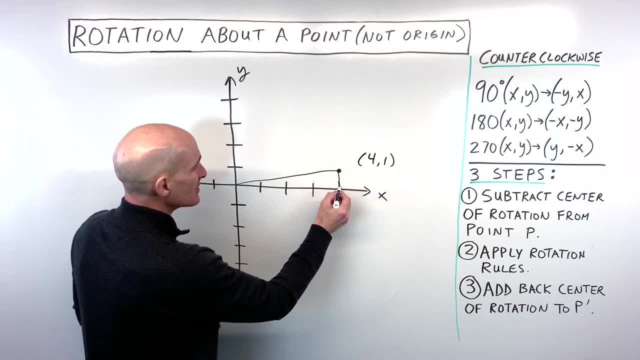 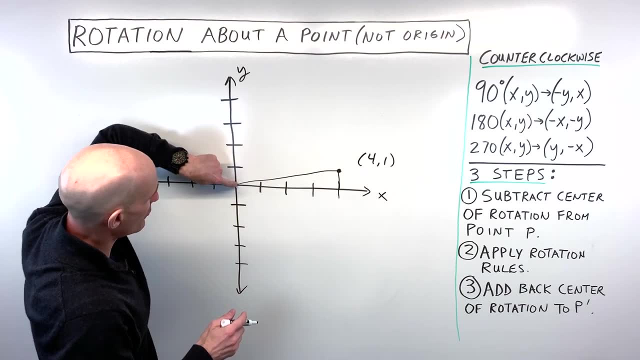 So visualize if I make a triangle like this. Okay, and so what we're going to do now is we're going to rotate this 90 degrees. So imagine if I held my finger right here at the origin And if this was on a sheet of paper, if I actually turned it 90 degrees, a quarter turn. 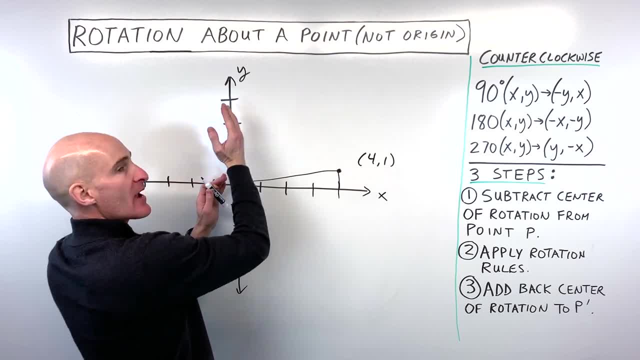 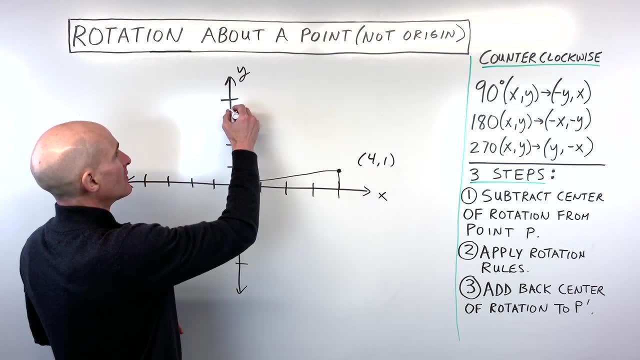 Well, what would happen is this x-axis would turn and match up with the y-axis, right? So what I'm going to do is I'm going to take this triangle, I'm going to rotate it, And so that's going to look like this now. 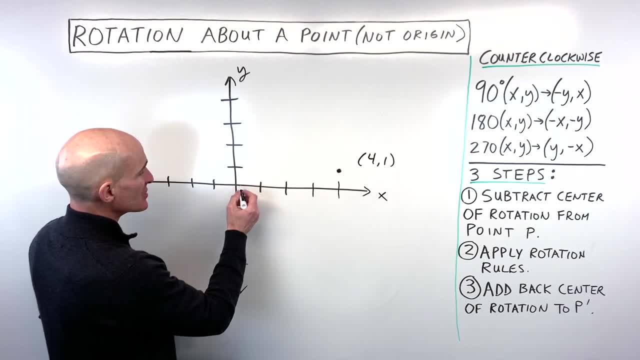 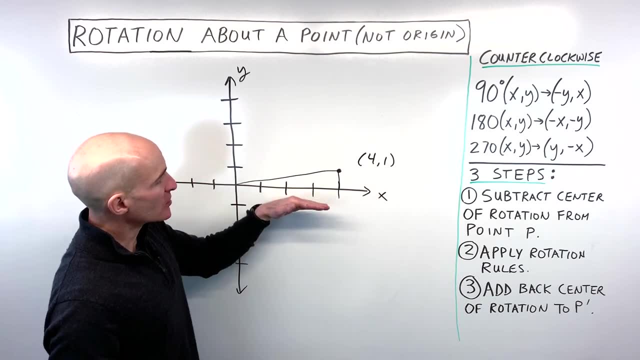 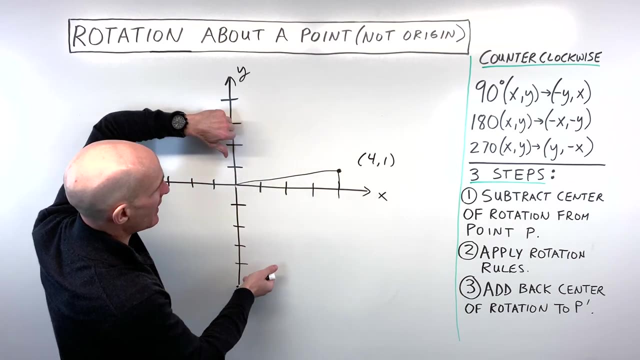 For one, what I like to do is just kind of draw this as a triangle. So visualize if I make a triangle like this. Okay, and so what we're gonna do now is we're gonna rotate this 90 degrees. So imagine if I held my finger right here at the origin and if this was on a sheet of paper, if I actually turned. 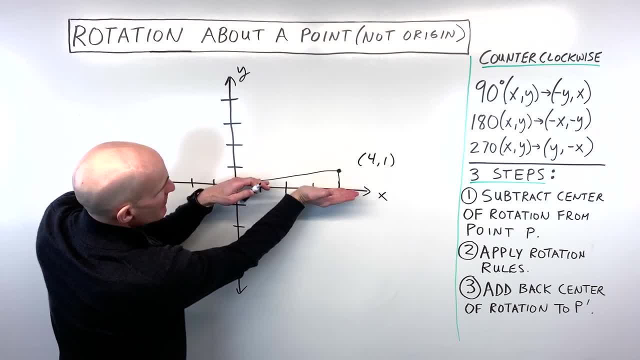 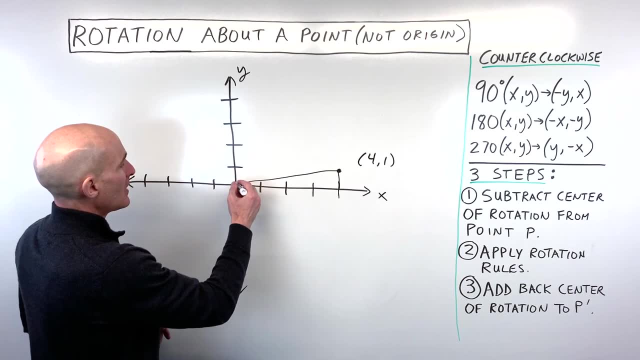 It 90 degrees a quarter turn. Well, what happened is this x-axis would Turn and match up with the y-axis, right? So what I'm going to do is I'm going to take this triangle, I'm going to rotate it, and so that's going to look like. 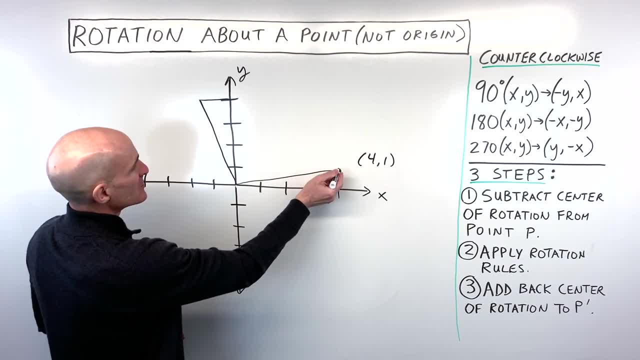 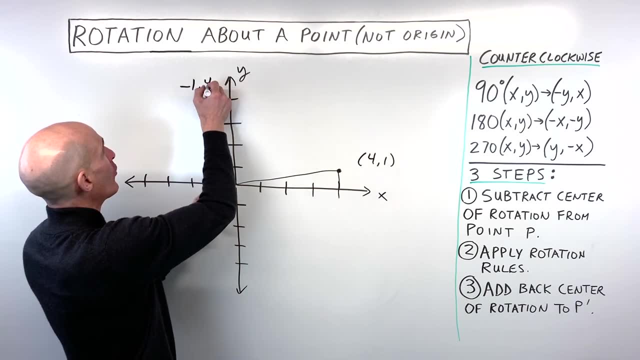 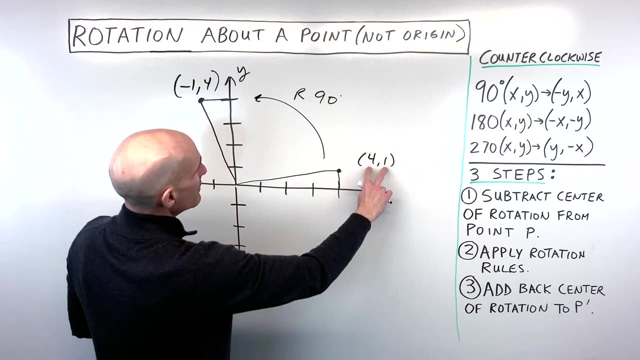 This now. Okay, so can you see it? So this point here will actually end up right here. And what is the location of this point? It's negative one, See left one up four. So when we rotated 90 degrees, What happened? Well, you can see that the X and the y-coordinates 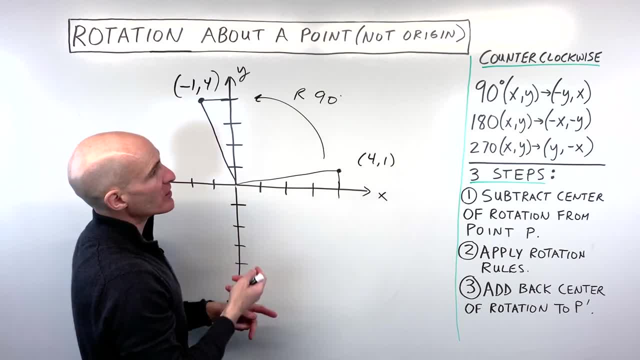 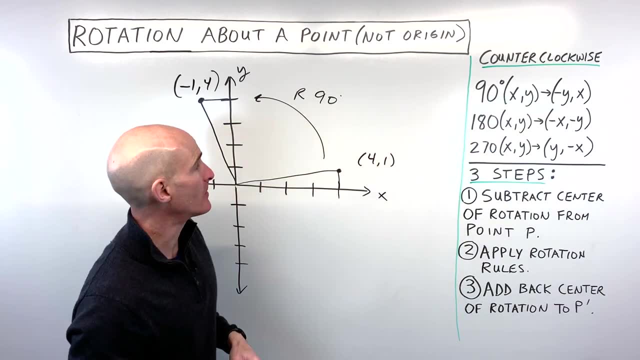 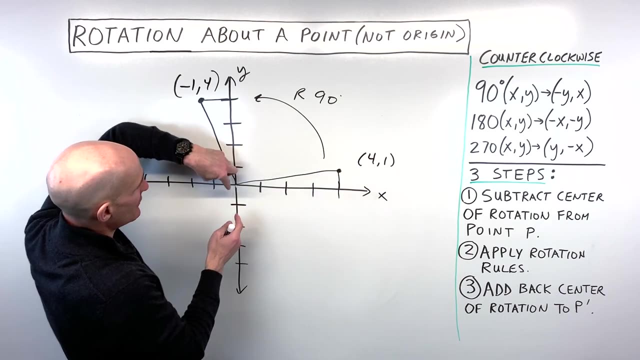 switched, But this new x-coordinate is the opposite sign. So see, we switched the x and the y and we made that new x the opposite. right now, Let's say, if we're going to rotate 180 degrees, so take this guy here 180 degrees. Imagine if I was holding my finger right at the origin here and I noticed a pivot or turn about this point. 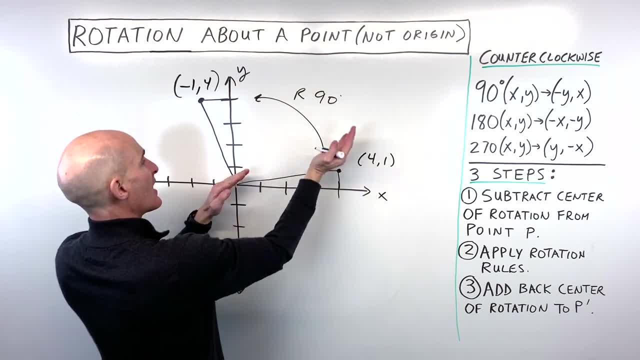 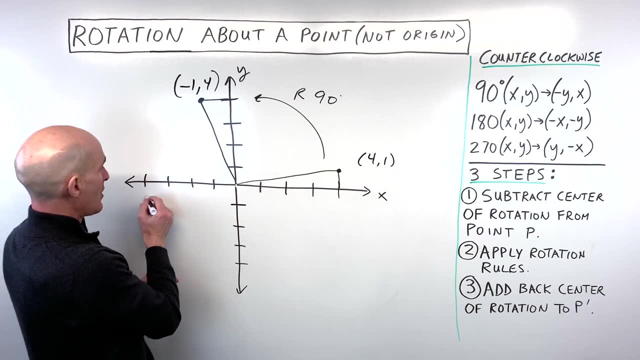 it would be like an surprises triangle by five degrees now і a half turn. so basically we would be rotating a half turn like this, and you can do this on a sheet of paper to kind of visualize, and so this would put us somewhere right about here, our triangle. 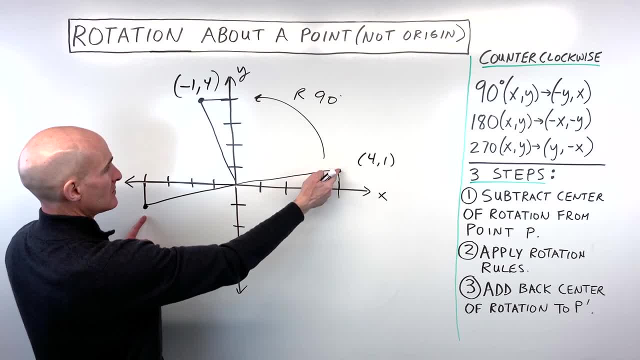 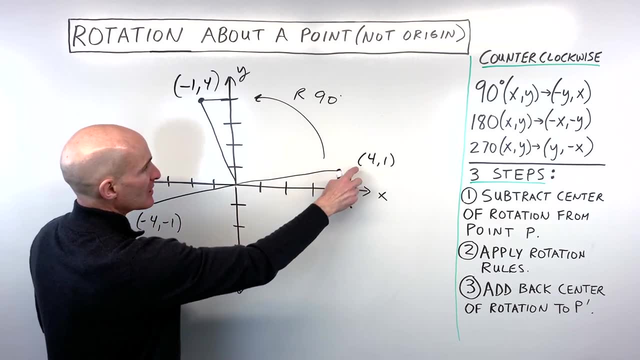 okay, and so you can see that this point. notice how this is like a straight line turning at a half turn. so this point is at negative four, negative one. now what happened here? from our original point, the x and the y are in the same location. four and one. it's just that the signs 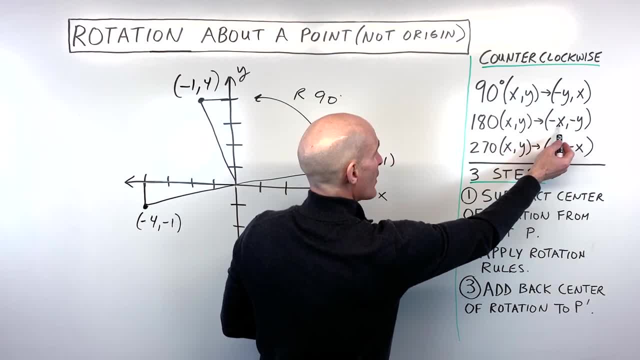 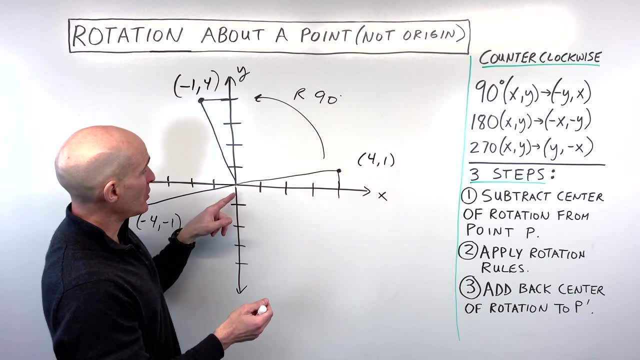 are the opposite. so see x and y negative, x negative y- same order, just the opposite sign. and then, lastly, if we were to rotate 270 degrees, that's going to be like a three-quarter turn. so i'm holding my finger at the origin, i'm turning my paper: 90, 180, three-quarters of a turn, that's. 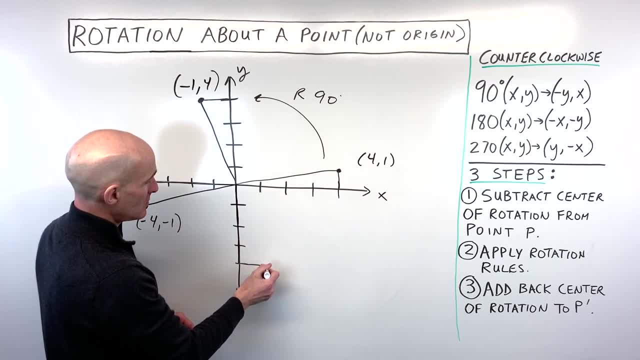 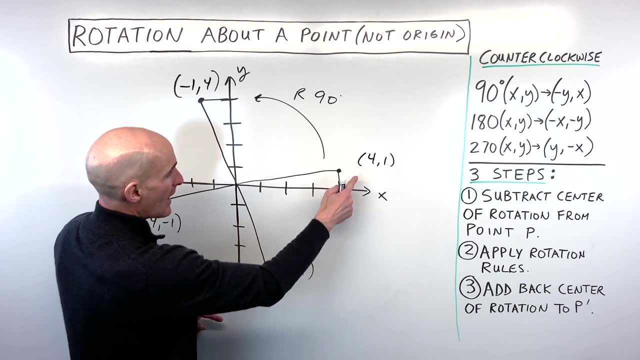 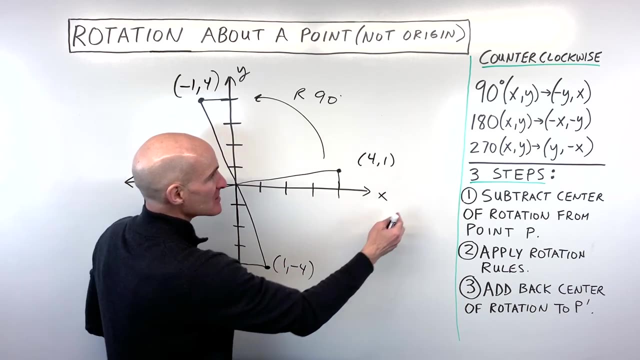 going to put us right here. and so there's your point. and that point is located at one negative four. what happened from this original point? well, you can, sweet see, we swear that's the opposite. so we're going to switch the x and the y right, and it's the new y, that's the 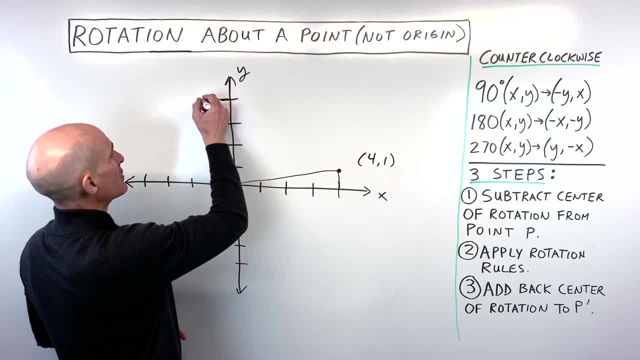 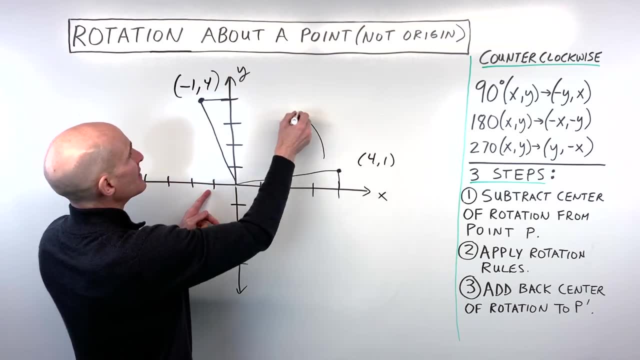 Okay, so can you see it? So this point here will actually end up right here. And what is the location of this point? It's negative: 1. See left. 1. Up, 4.. So when we rotated 90 degrees, what happened? 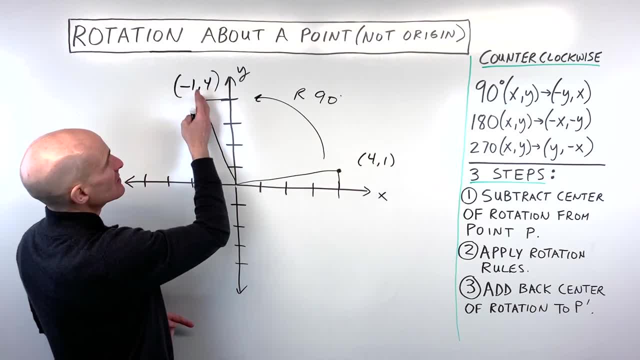 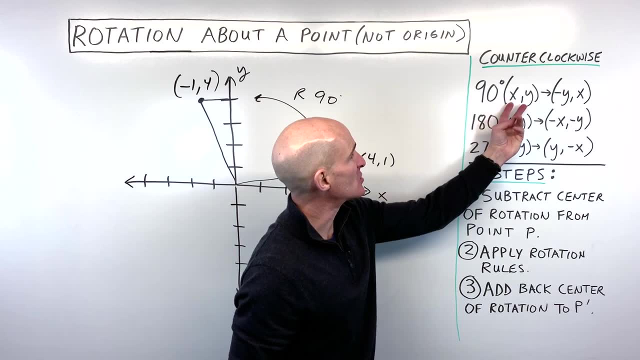 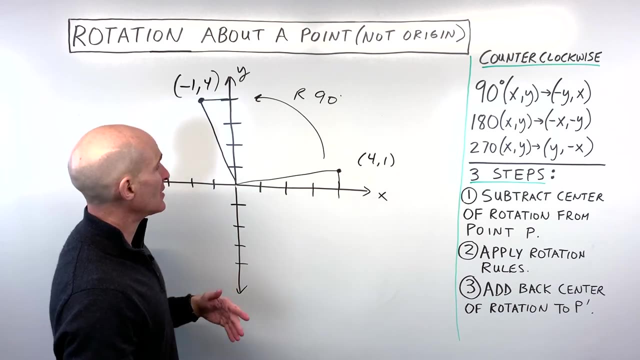 Well, you can see that the x and the y coordinates switched, But this new x coordinate is the opposite sign. So see, we switched the x and the y, We made that new x the opposite. right Now, let's say, if we're going to rotate 180 degrees, 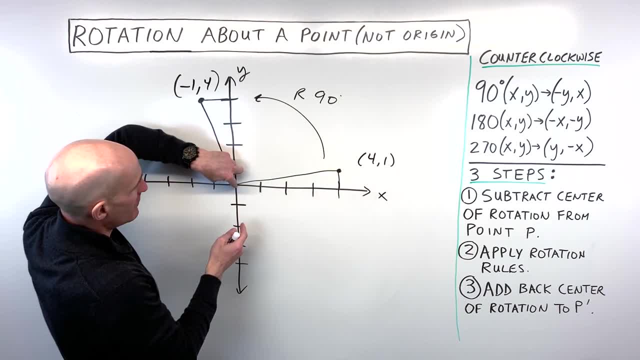 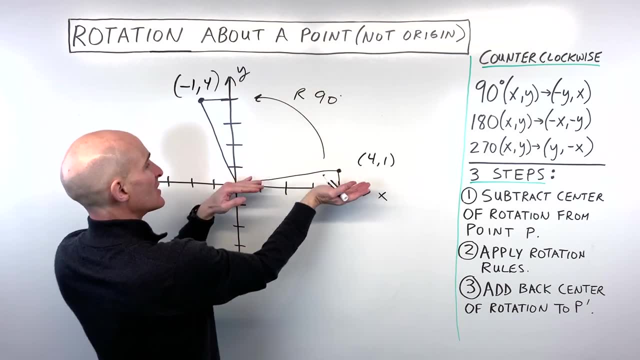 So take this guy here, 180 degrees. Imagine if I was holding my finger right at the origin here and I was to pivot or turn about this point. it would be like a half turn. So basically we would be rotating a half turn like this: 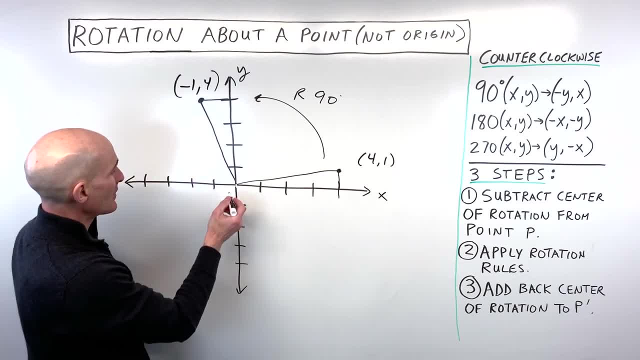 And you can do this on a sheet of paper to kind of visualize, And so this would put us somewhere right about here, our triangle, Okay, And so you can see that this point, notice how this is like a straight line, turning at a half turn. 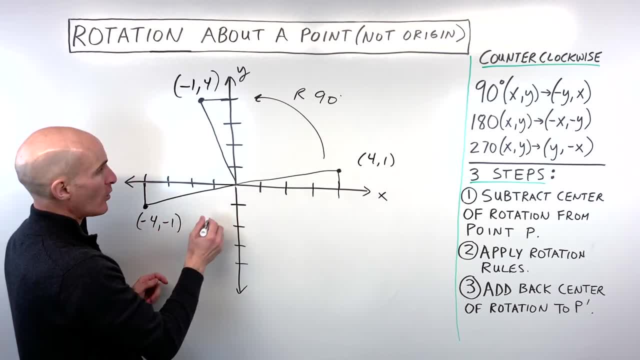 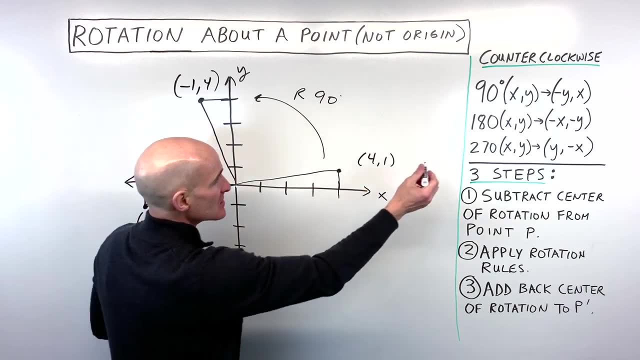 So this point is at negative 4, negative 1.. Now what happened here? from our right The original point, the x and the y are in the same location: 4 and 1. It's just that the signs are the opposite. 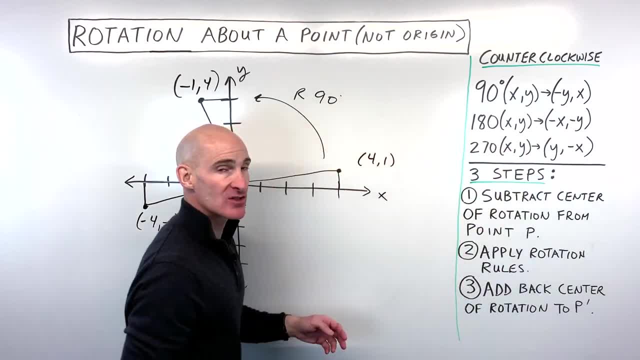 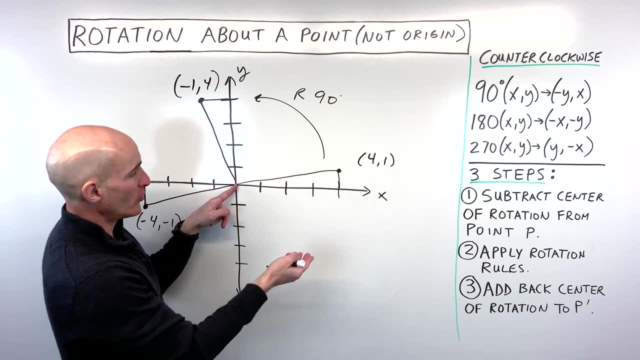 So see x and y negative, x negative, y- same order, just the opposite sign. And then, lastly, if we were to rotate 270 degrees, that's going to be like a three-quarter turn. So I'm holding my finger at the origin, I'm turning my paper: 90,, 180,, three-quarters of a turn. 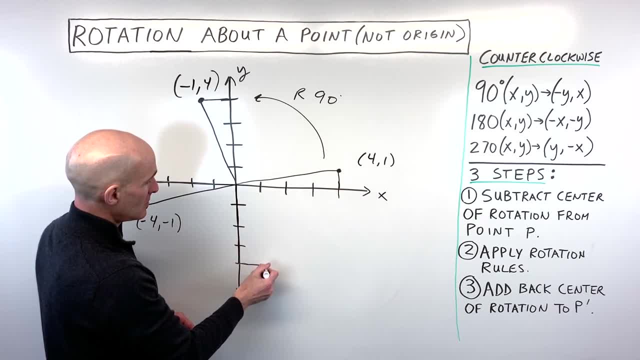 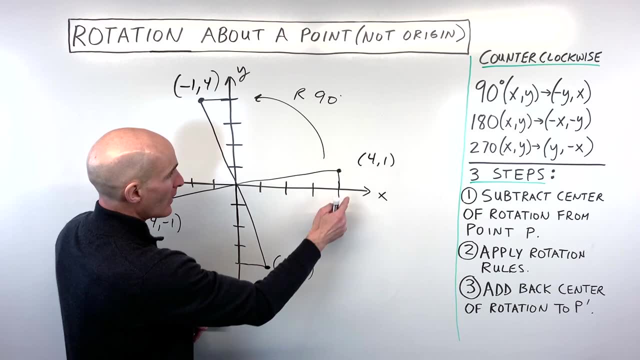 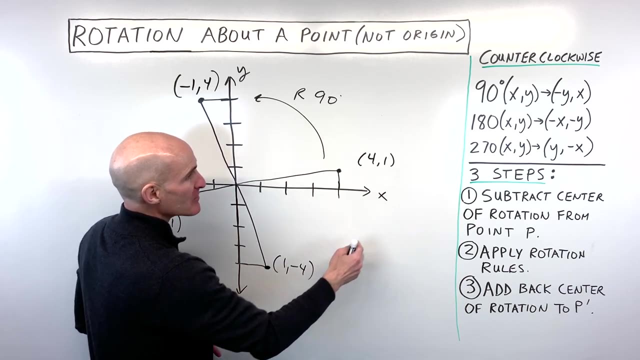 That's going to put us right here. And so there's your point, And that point is located at 1.. Negative 4, what happened from this original point? Well, you can see, we switched the x and the y right and it's the new y. that's the opposite. 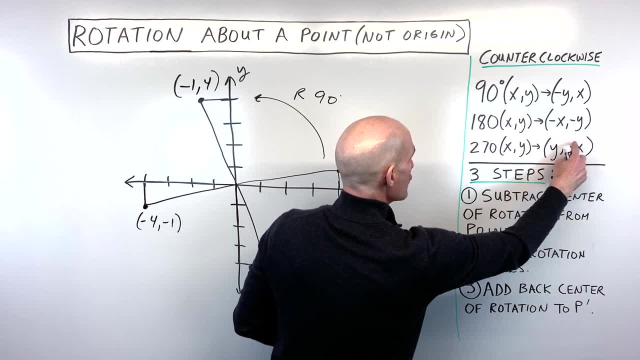 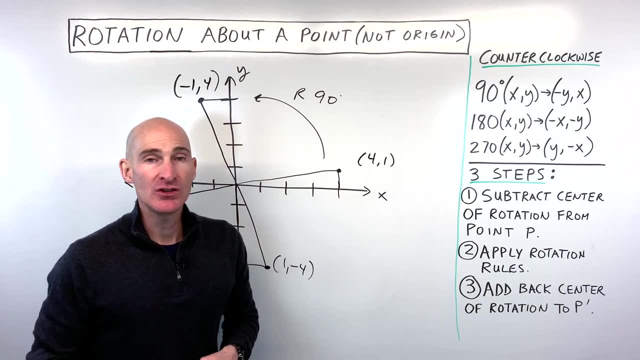 So see x and y are switching, see y, x, but it's that new y. that's the opposite. So that's how I like to think about it. Maybe that's helpful for you too, If you like the way that I explain things and you want to learn more about Algebra 1 or Algebra 2, college algebra.